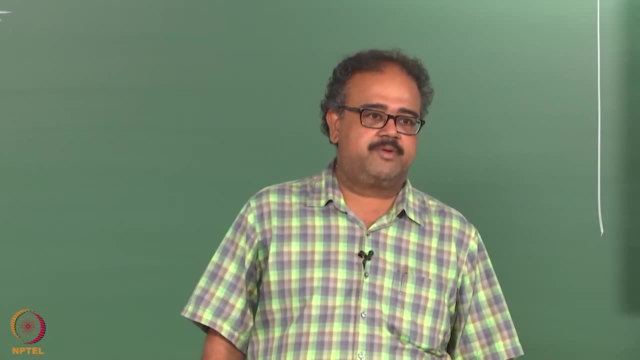 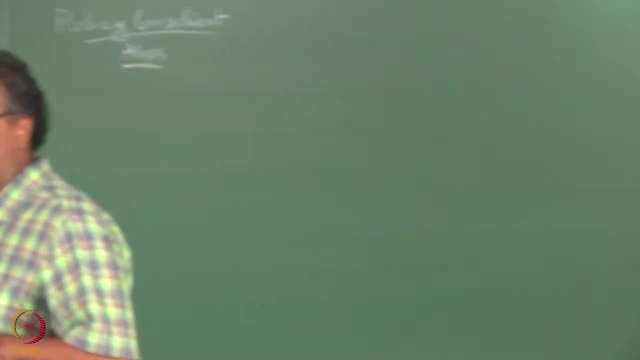 terms of the distribution of the value over the state space than the policy. So the classical example I give for this is the inventory control problem. So the inventory control problem, essentially the policies that you will be considering, are what are called threshold policies. If 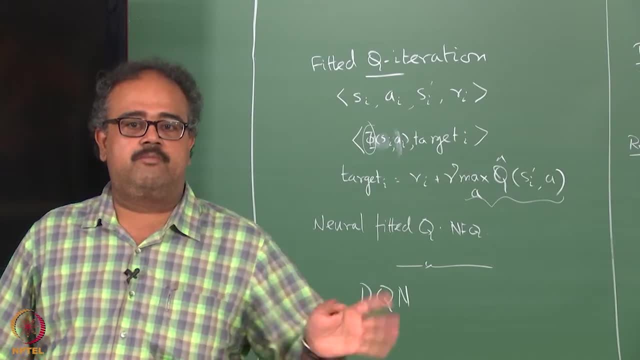 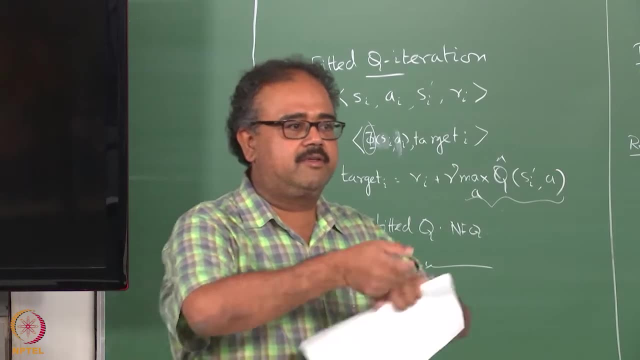 the inventory is below x, you buy. If the inventory is above x, you do not buy. So that is essentially what it will reduce to. The policies will reduce to that. But if you look at the value function, so depending on some kind of a cross product of what are all, 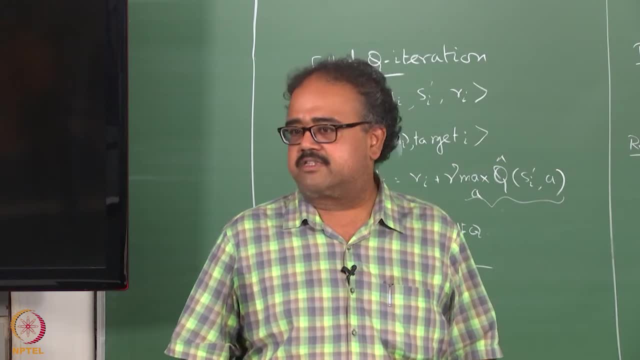 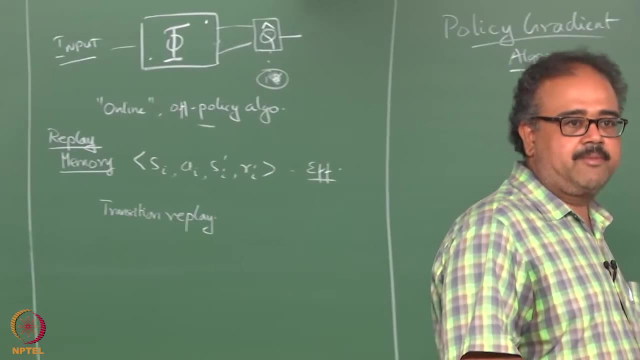 the things that are available, you will get some very complex function, depending on how the rewards are worth and so on and so forth. So from a representation point of view it is lot easier to represent policies in some cases than it is for. 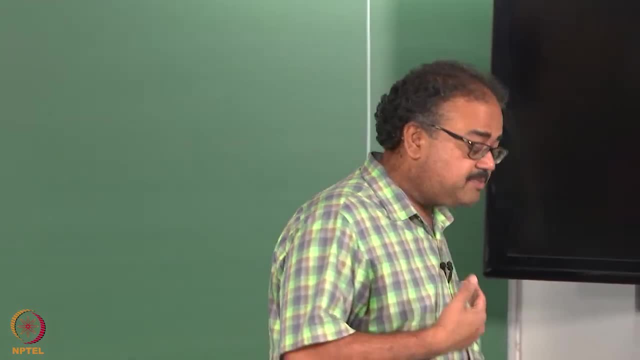 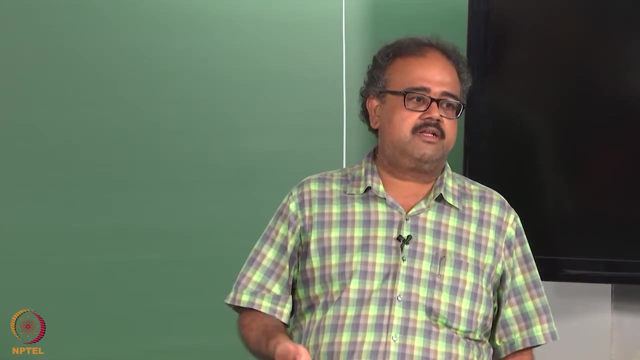 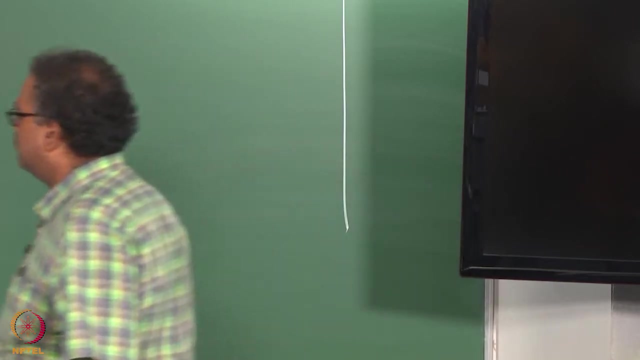 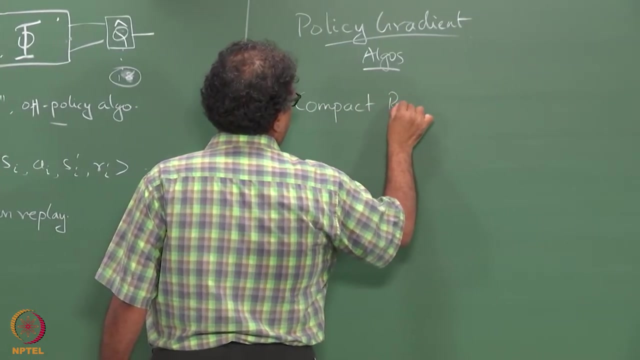 Now how you are itemized to represent currencies. So you have different kinds of染iders and patterns, As I will discuss further. you will see in the next lecture. in this entire lecture, five for all non-family of often. 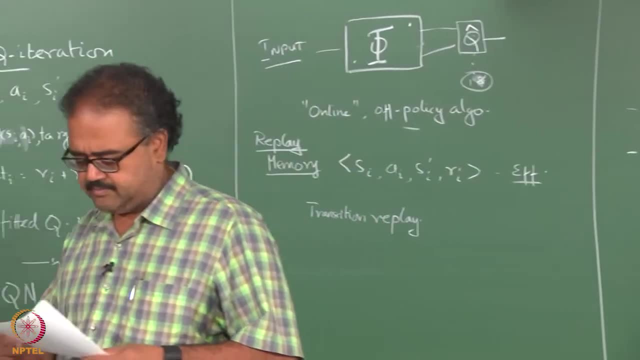 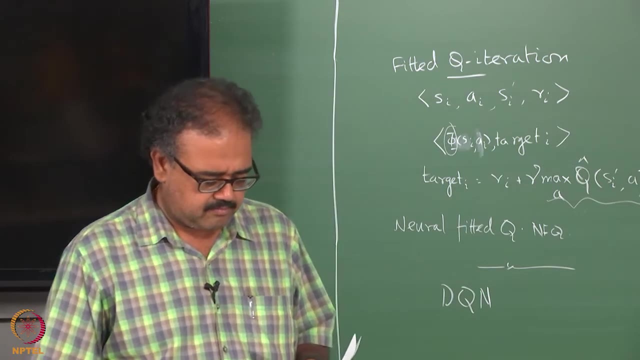 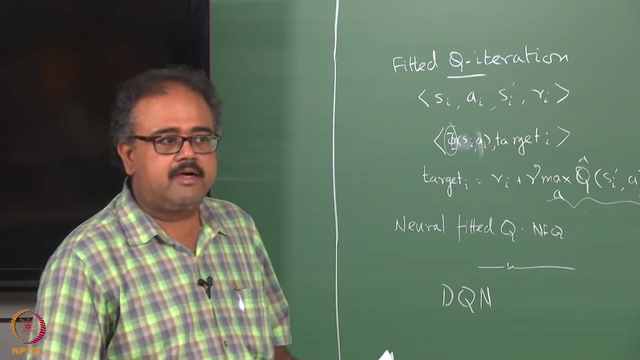 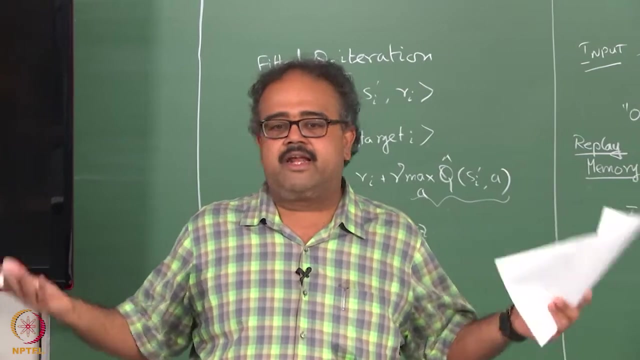 Of features, All types of features. What do you think is the second advantage, Again, when we move to the parametrized forms, right, so value functions, value function, approximation methods, right, are not guaranteed to converge anymore, right? I mean, they work fantastically. So we have dqn and other things. 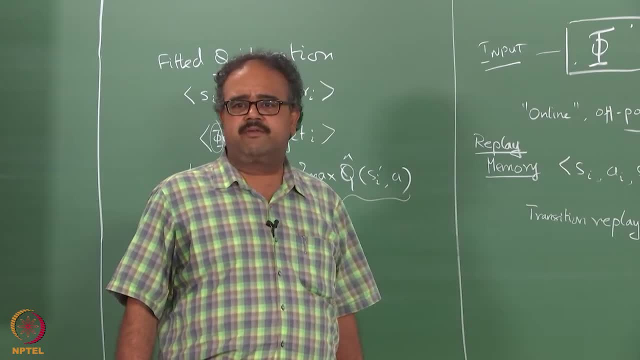 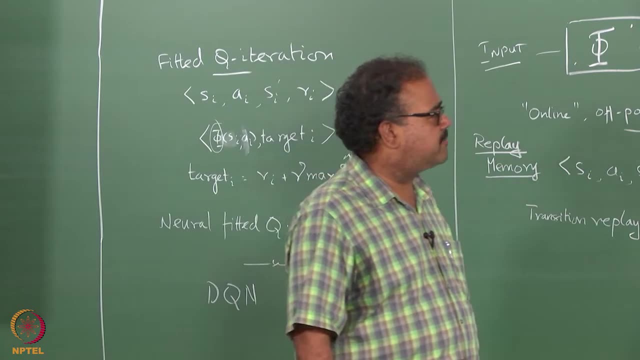 but you really do not have much of a intuition as to how they will converge, except in the case of linear function, linear parametrization, right, And it is not 100 percent clear how things will work. But in the case of policy, gradient algorithms. so you have some kind. 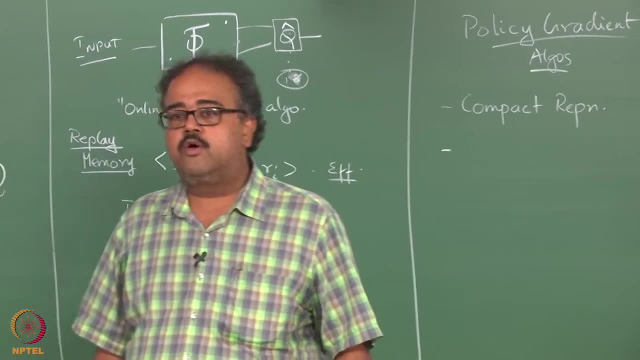 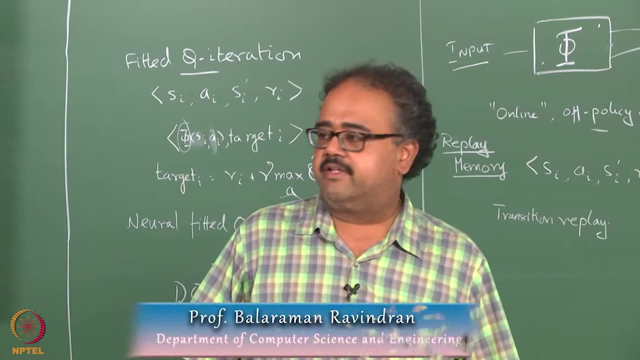 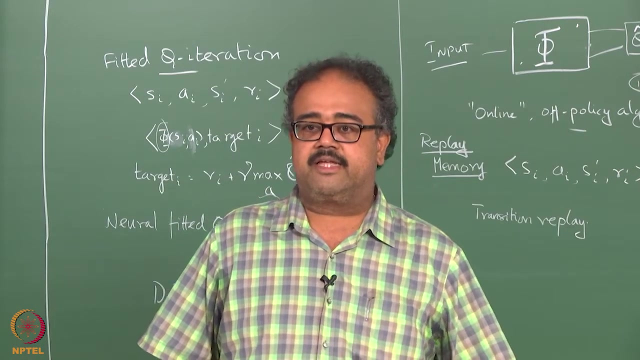 of guarantees that they will at least converge to local optimum, right, And so that seems to give us a lot more leverage, right, in the sense that you can say, oh, things will be stable, You know, if I keep running this for some time, it will converge to something, right? 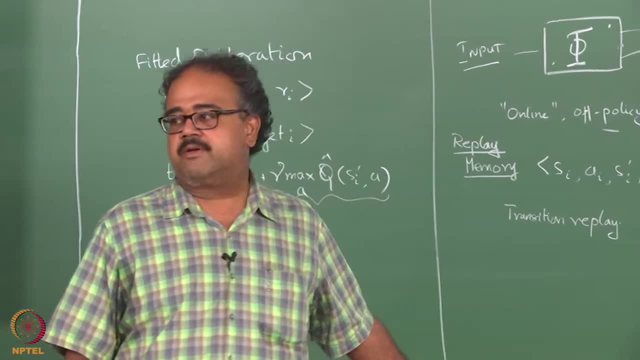 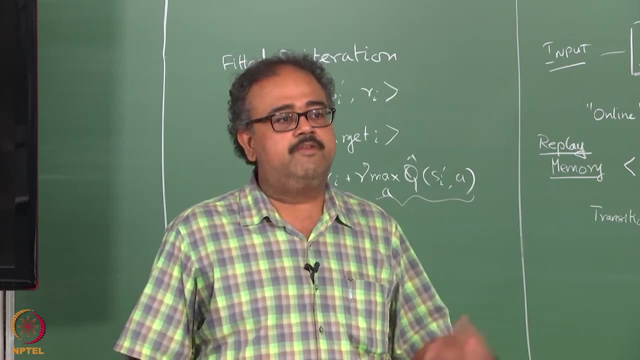 In the case of value function methods. I do not know, It might even diverge right, It might start oscillating. So I have no guarantees as to the behavior of the methods under value function approximation. So when I am working with really large problems it might be better. 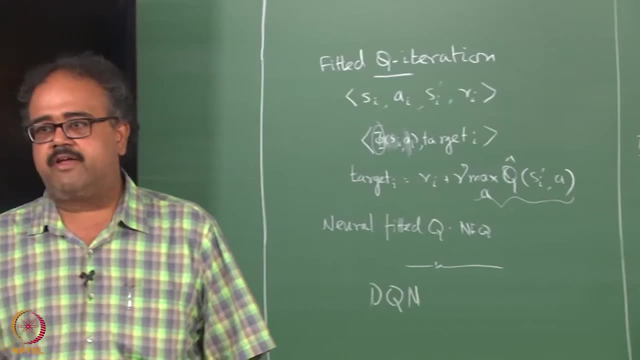 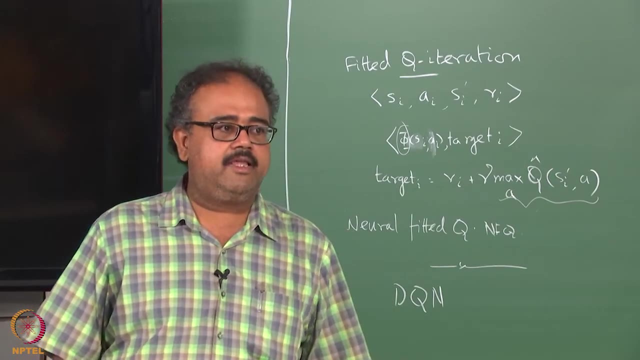 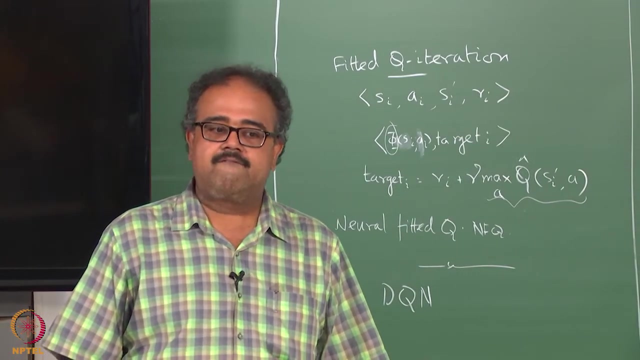 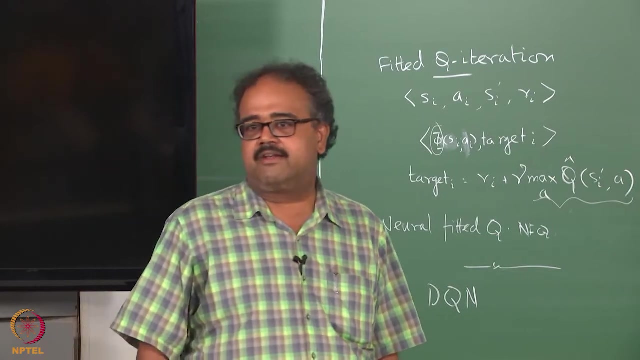 off working with policy approximations than with value function approximations- okay. Having said that, I should also point out that almost all the large scale successful applications of reinforcement learning right have involved value function approximations. okay. So in theory it does not guarantee to work, but in practice it does seem to. 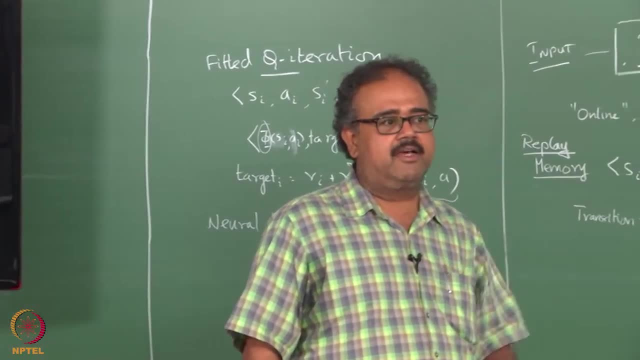 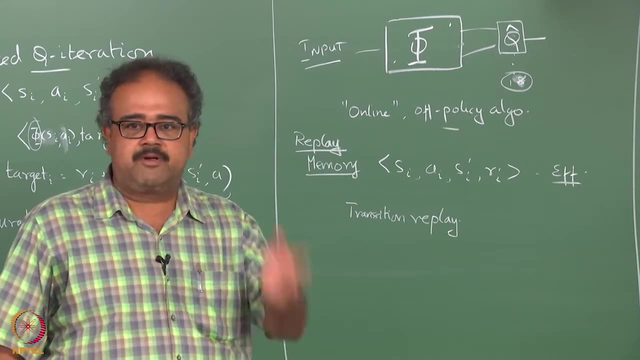 work. Of course, you can always come up with examples where things did not work, also in practice, right? So you can always come up with very, very simple examples. like people talk about XOR killing neural networks- right? So you can always come up with very simple counter examples where you can show that. 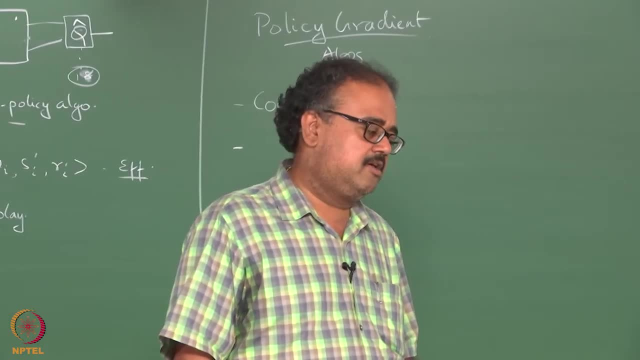 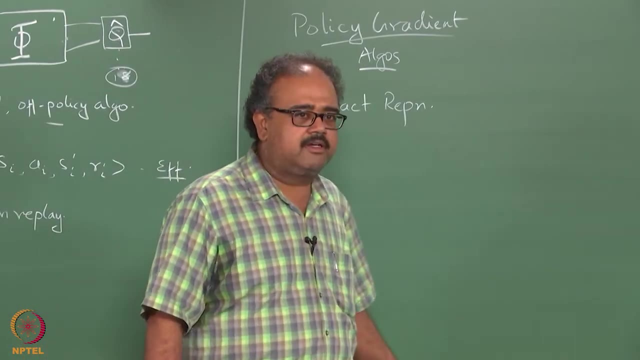 approximation is really not going to converge. Therefore, people are always a little wary about doing neural networks and other things until deep mind came along and now everybody does neural networks. So if you now try to write a reinforcement learning paper without deep networks in it, 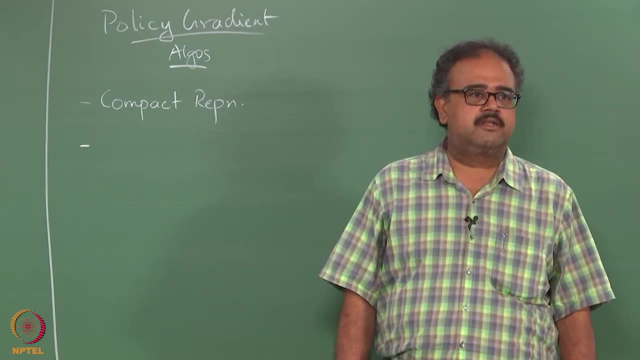 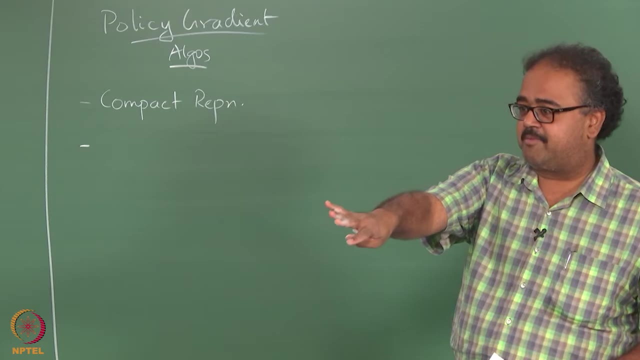 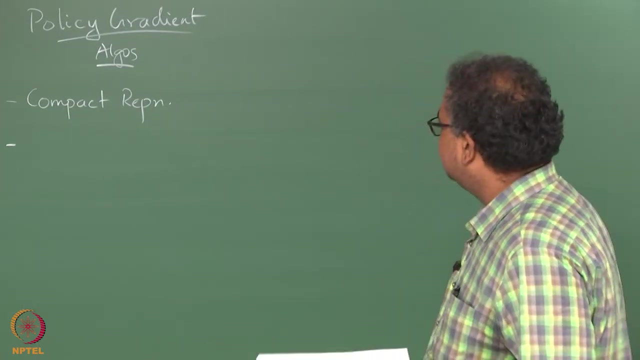 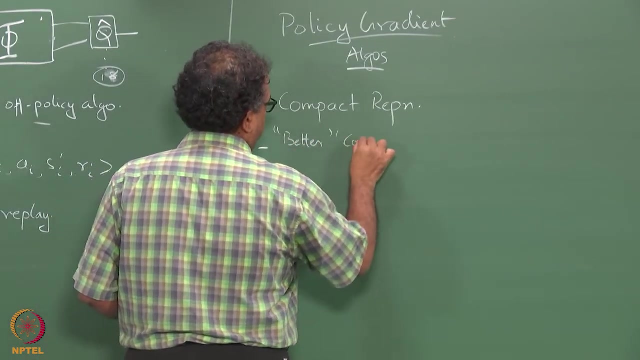 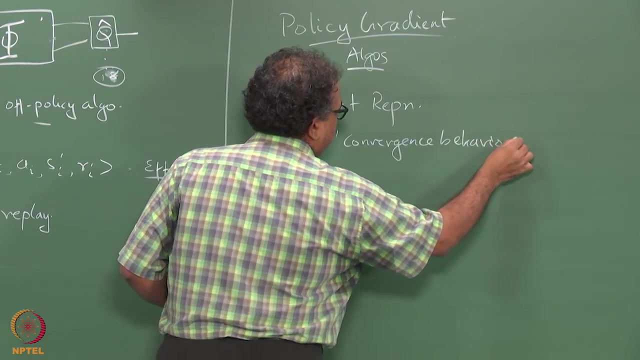 immediately, your chances of getting accepted goes down by 20 percent. so that is how the times have changed, Of course, except if you write banded papers. So banded papers do not need deep networks in it. The second thing is- I am going to put this in quotes- where the convergence behavior 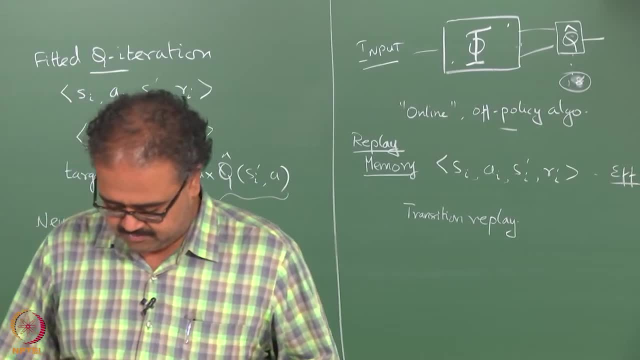 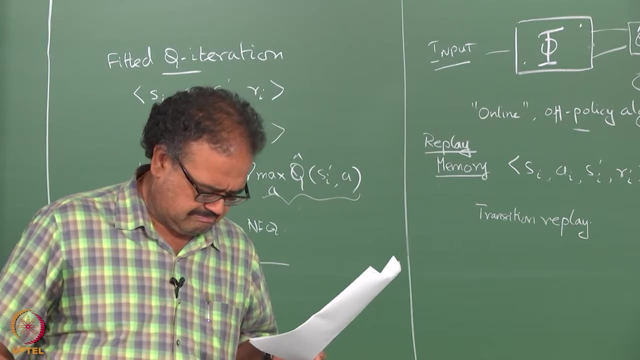 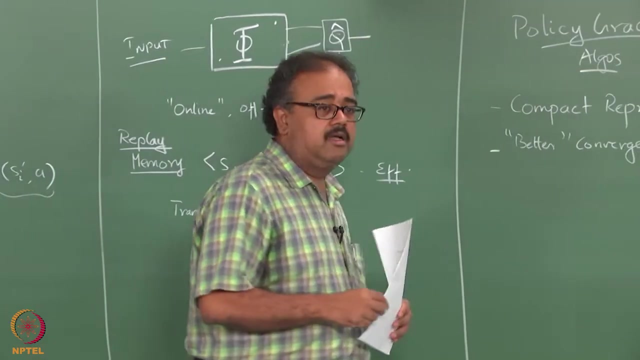 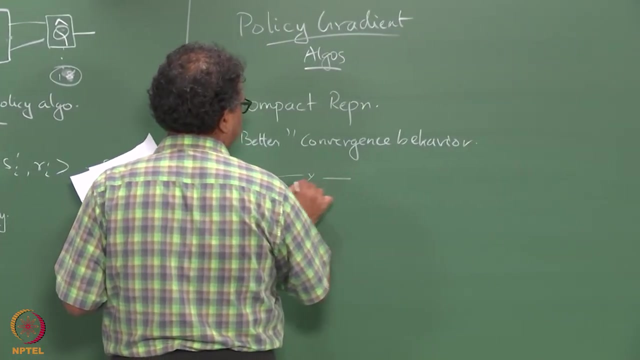 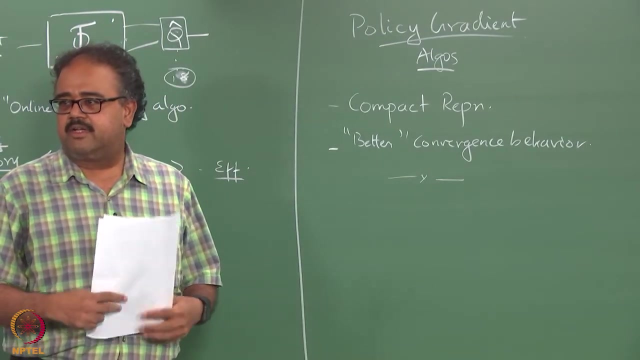 is. So what do value functions, what do policy gradient methods do? So you actually have some kind of a- I put better within quotes because it is, I mean in practice. value function based methods also seem to work with the functional approximation. 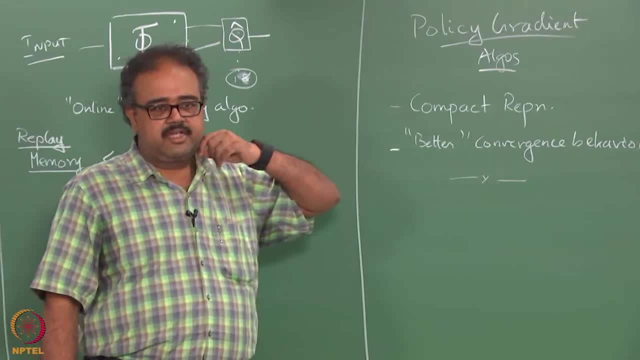 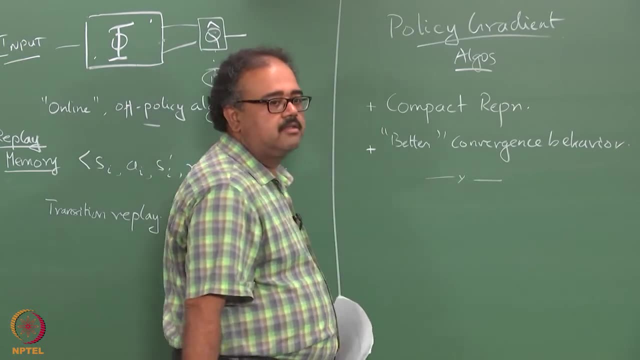 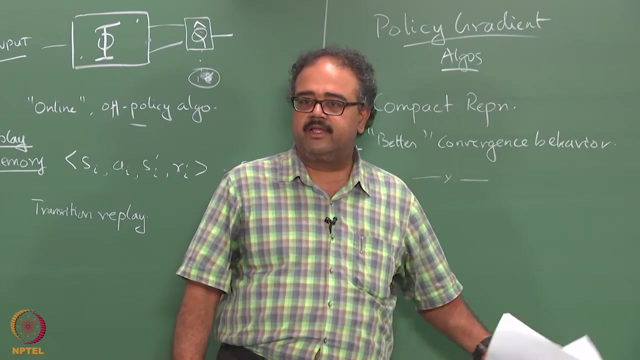 but policy gradient you can actually give some kind of a guarantees about it. So what are the problems with policy gradient approaches? We will come to that in a bit. so after I describe what we are doing, then I will ask you some questions and then you will know what the problems are. 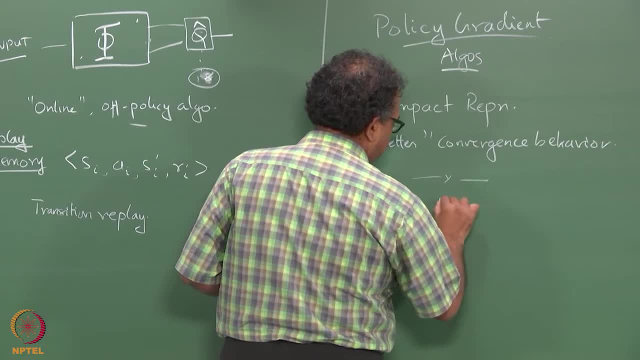 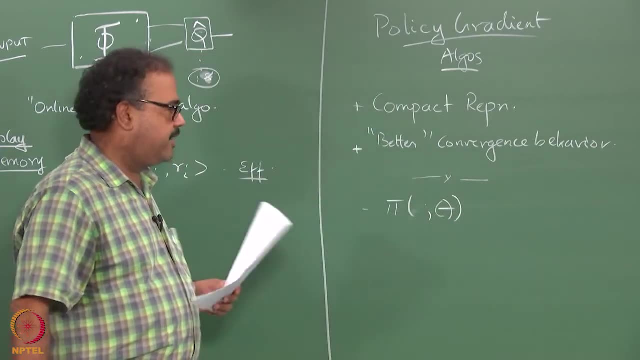 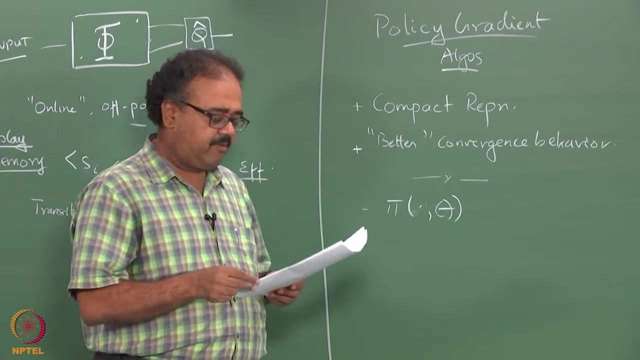 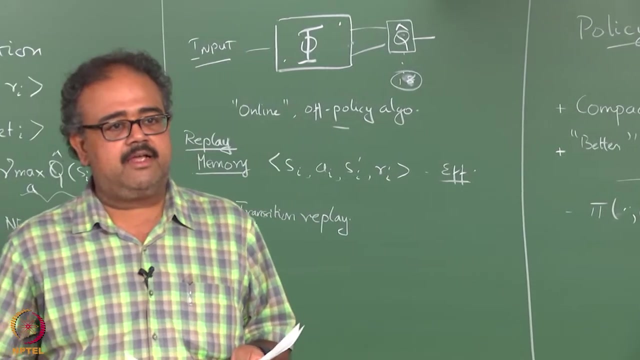 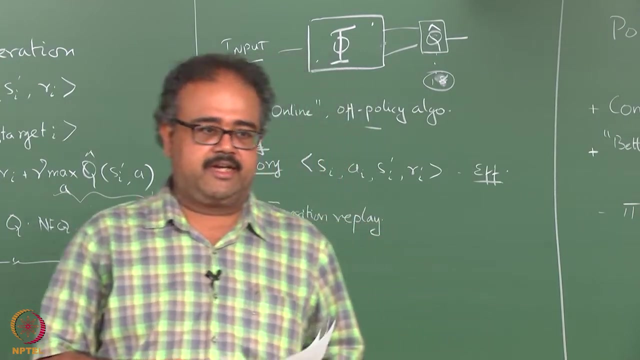 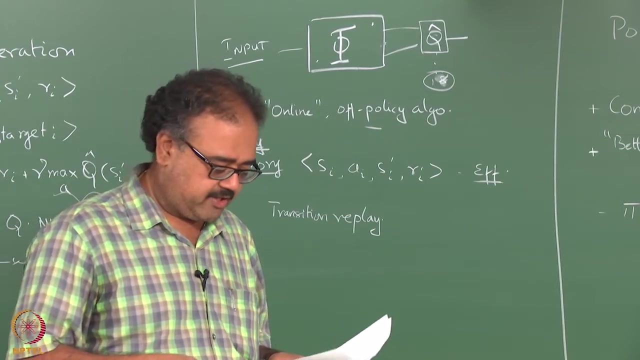 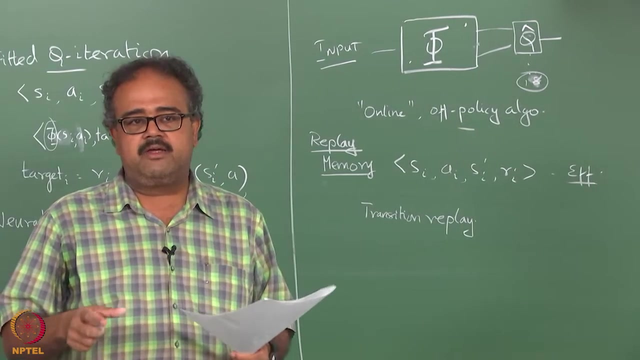 So essentially, you are going to say my policy pi depends on some set of parameters, theta, so I am always going to write this as right. And so then now let us gradient descent. we all know that it will eventually reach a global or local optima, under certain conditions, right? 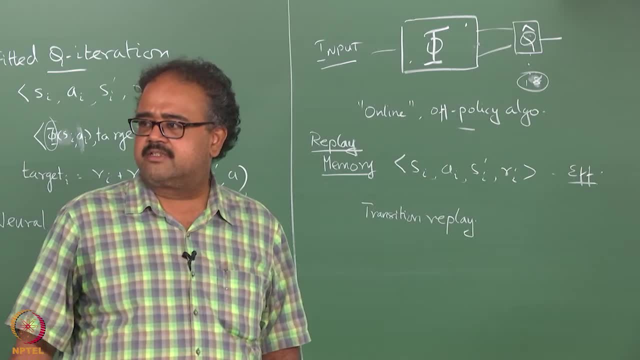 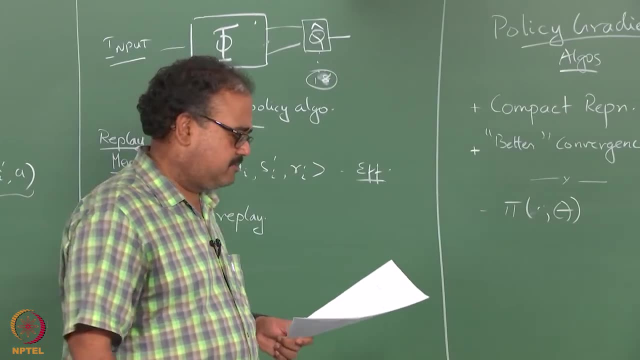 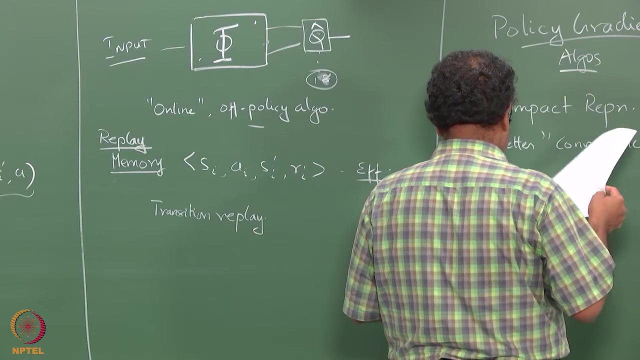 So you have to make take small enough step sizes and there are small conditions on the step sizes. and then you are: gradient estimate should be unbiased, or at least biased favorably, and so on, so forth, right, So if you remember, 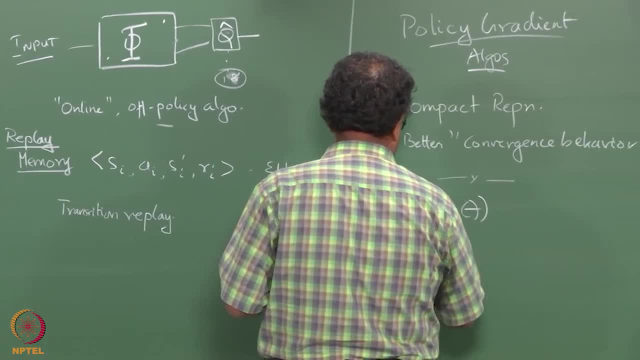 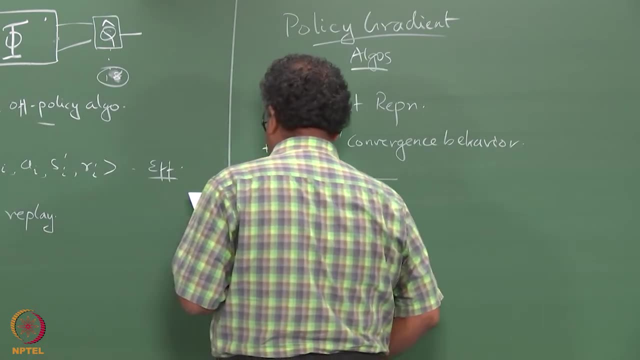 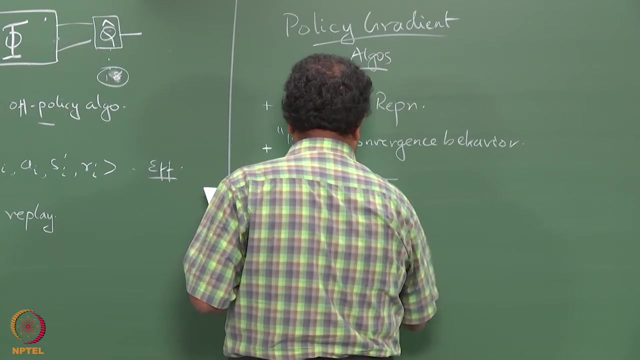 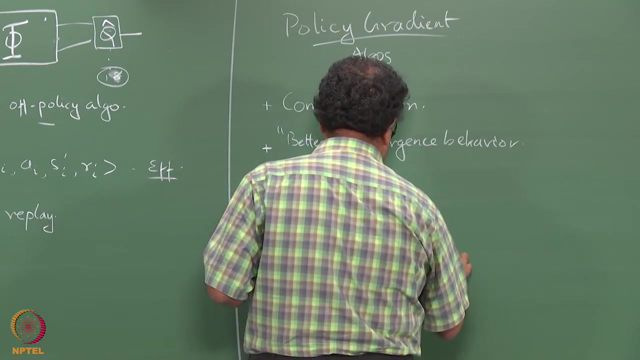 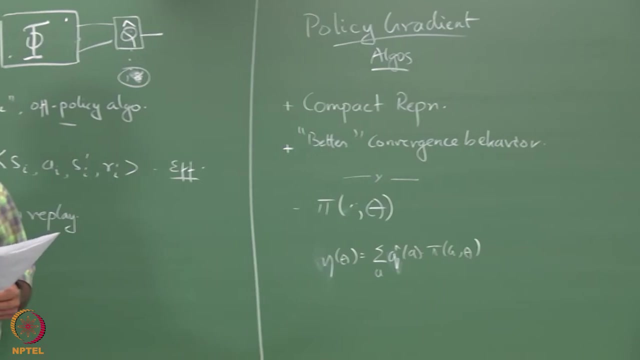 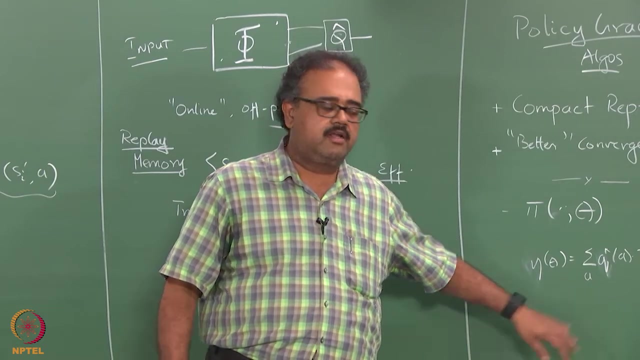 So we essentially talked about the- this is from the reinforced lecture- right? So we kept that as the performance measure, right So which, of course, we could not estimate directly because we did not know q star. right So we did not know q star, So we could not. 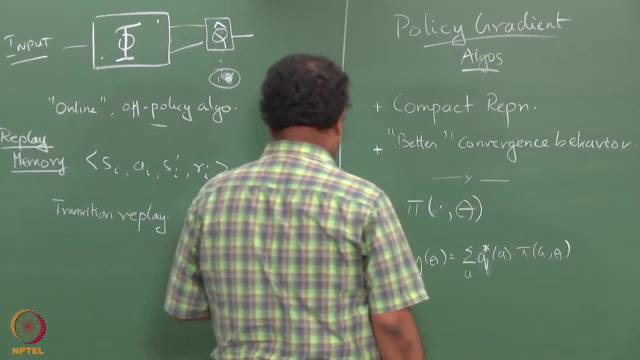 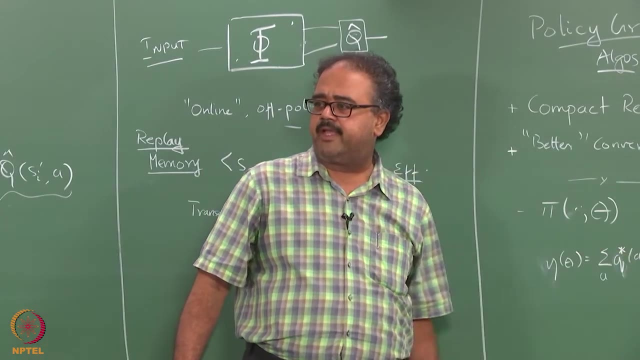 estimate this directly. So what did we do? We did a whole bunch of sleight of hand, right? So we divided this by, we took the gradients, divided it by pi, blah, blah, blah and finally we came up with a. 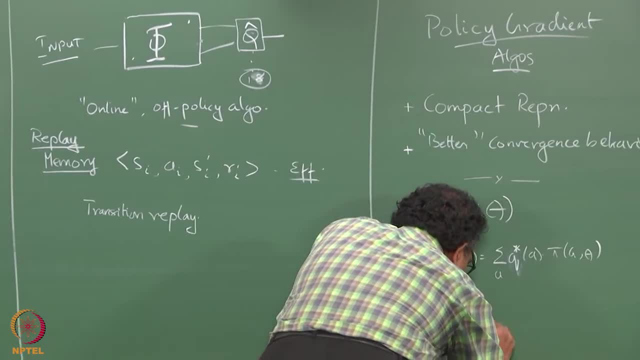 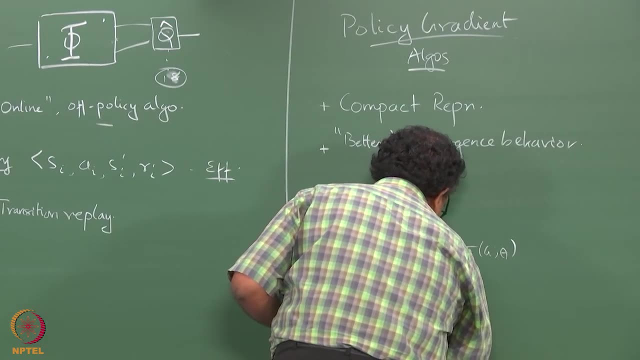 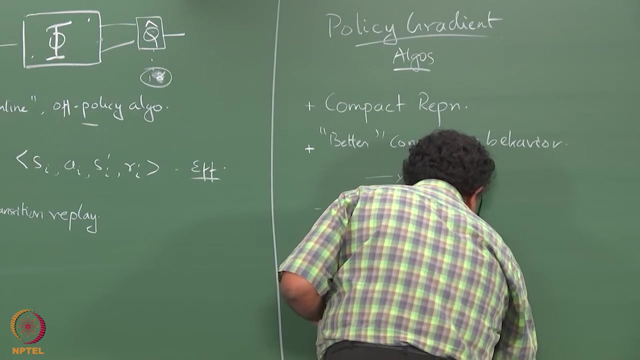 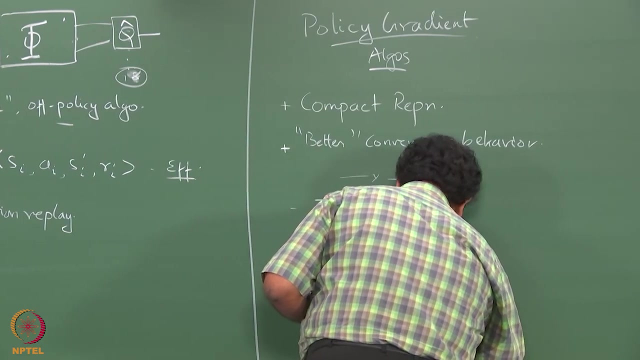 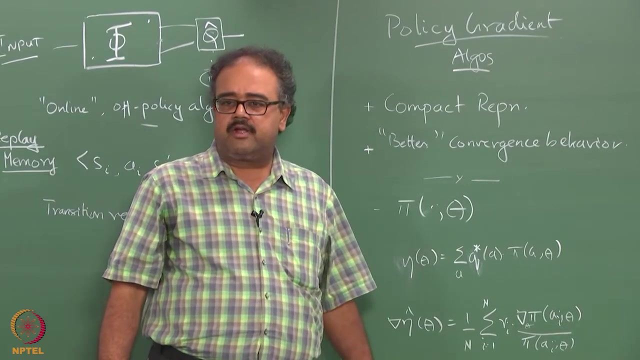 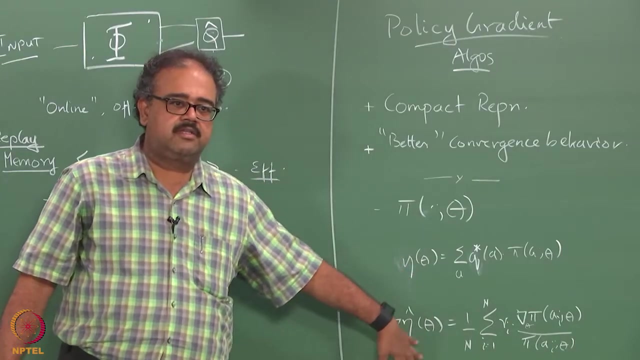 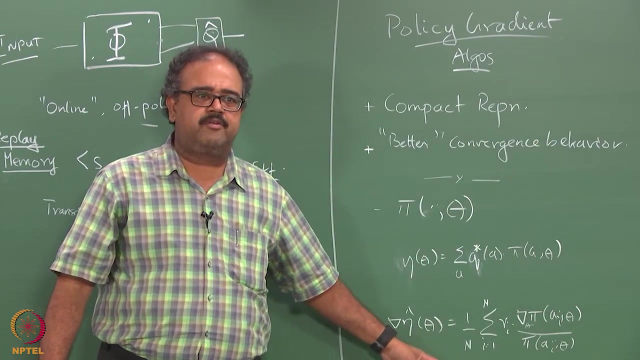 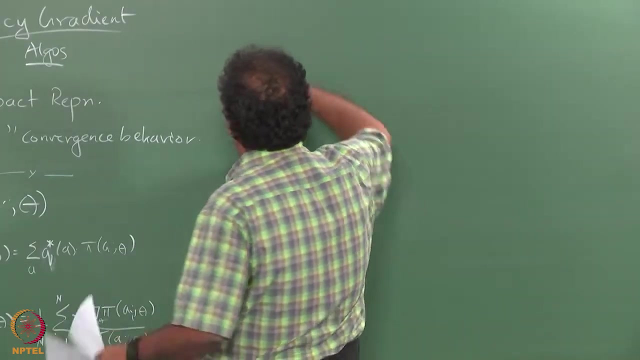 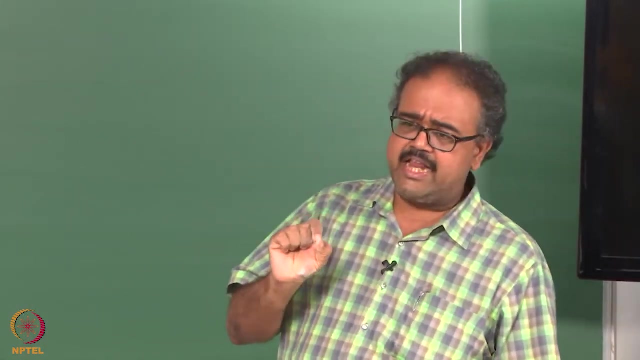 estimate for the gradient that looked like this: 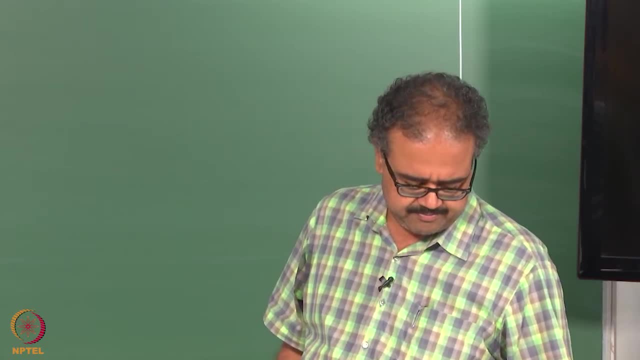 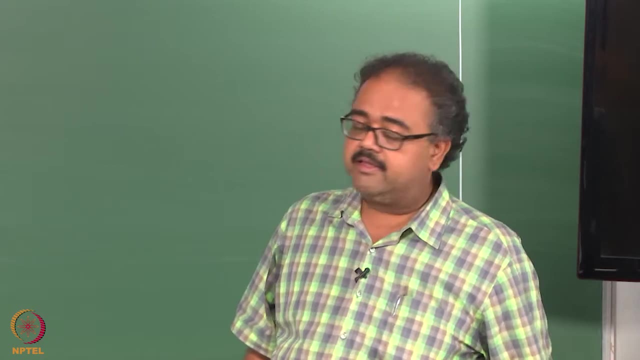 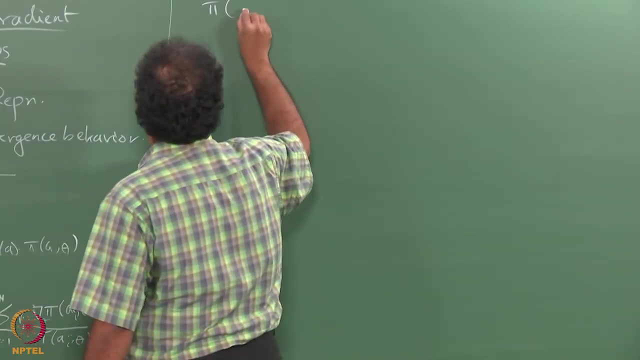 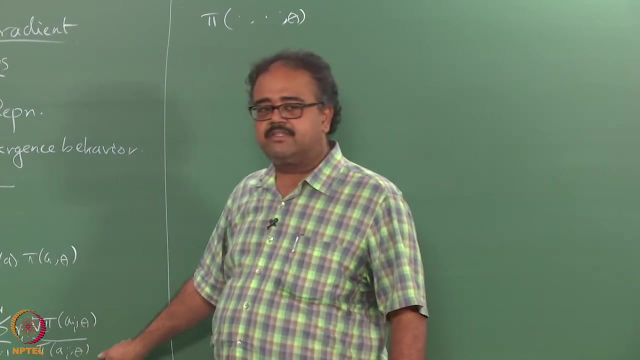 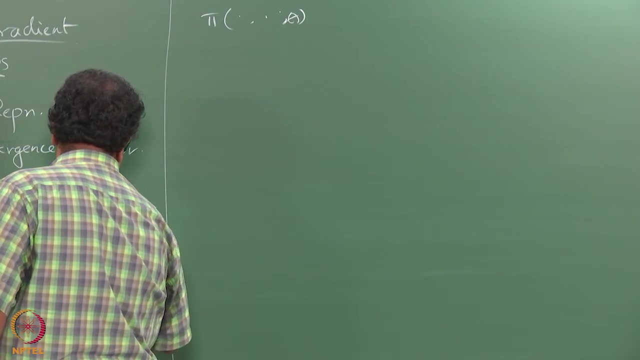 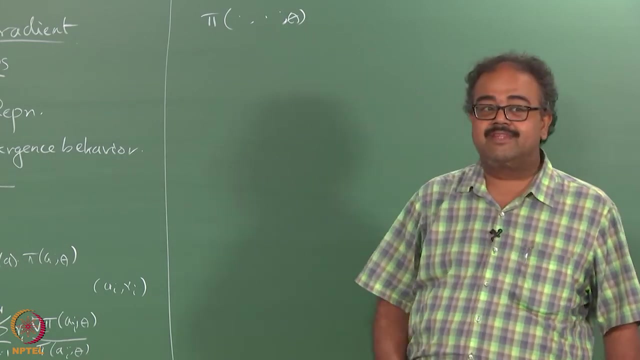 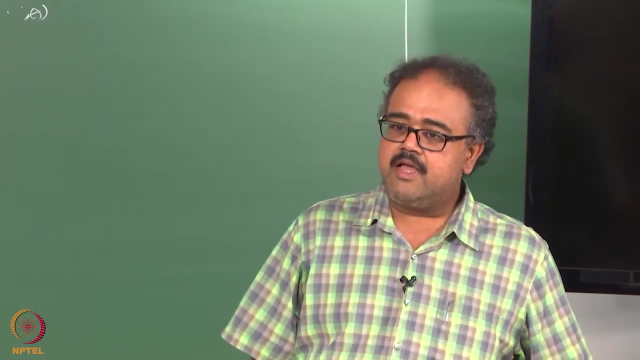 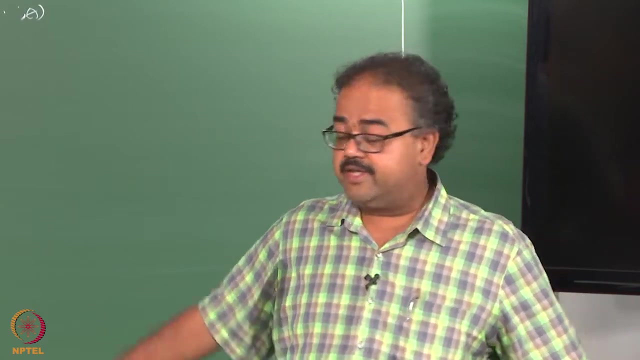 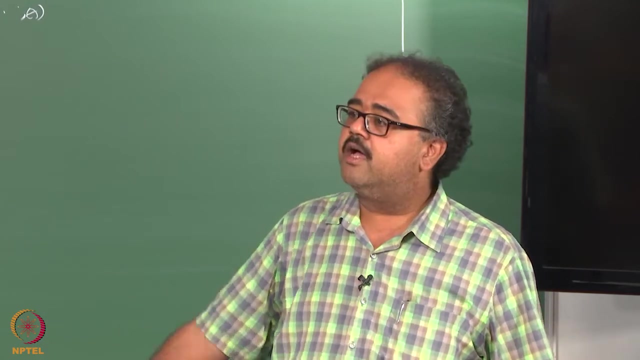 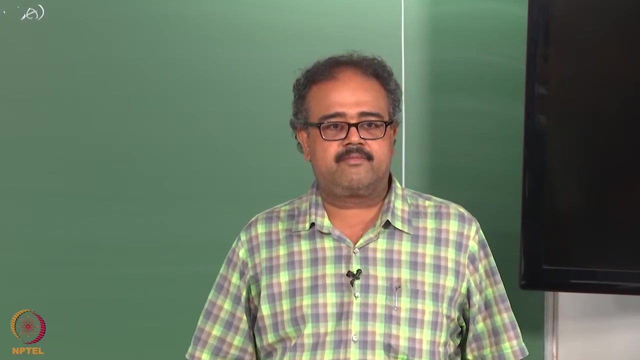 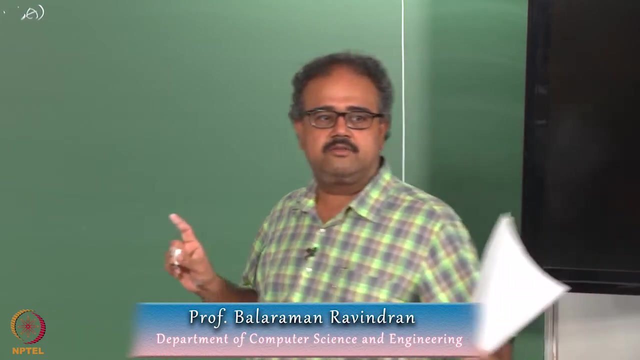 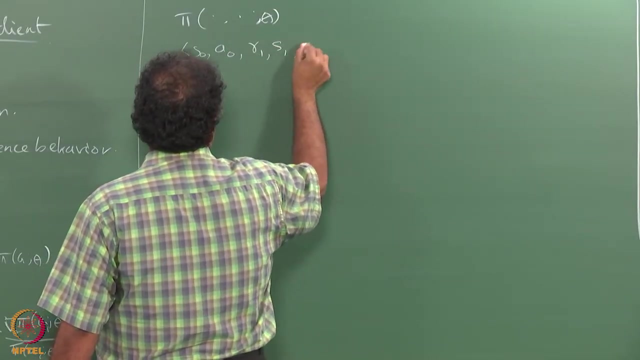 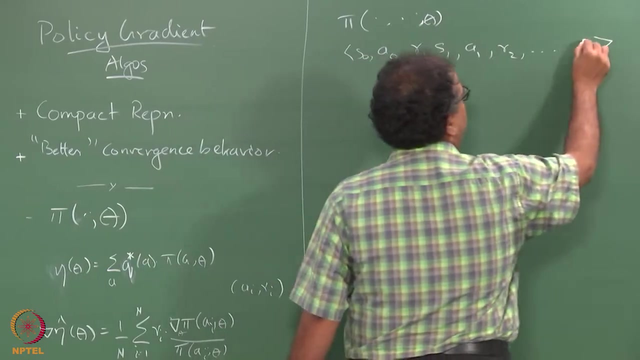 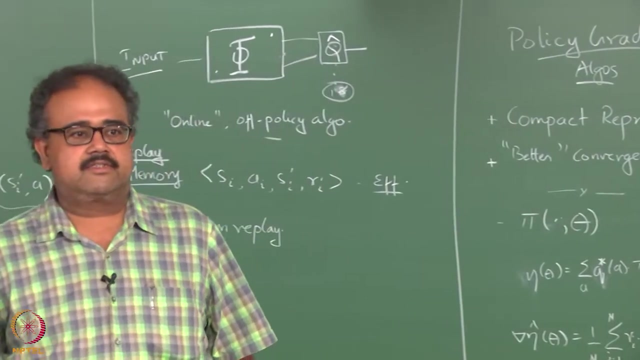 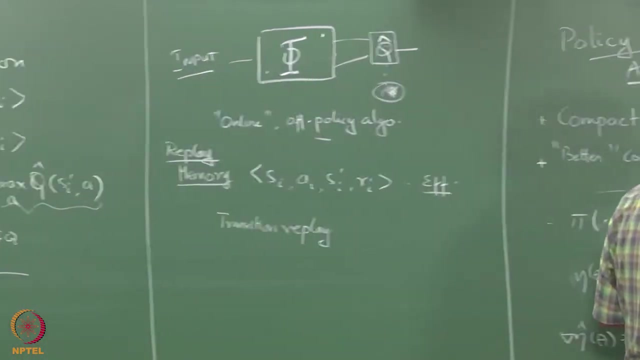 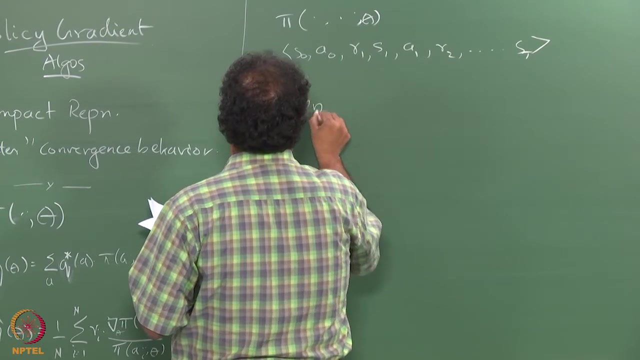 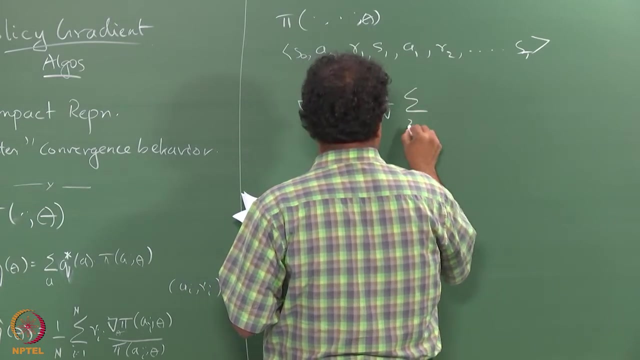 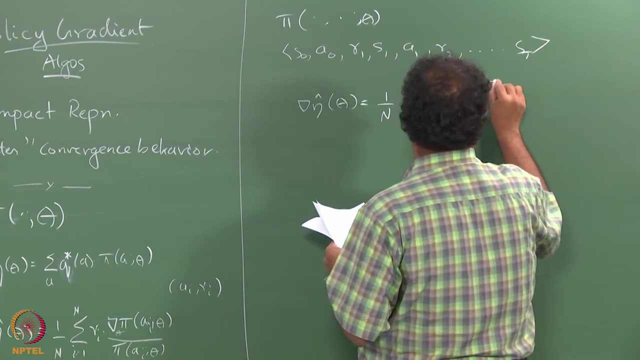 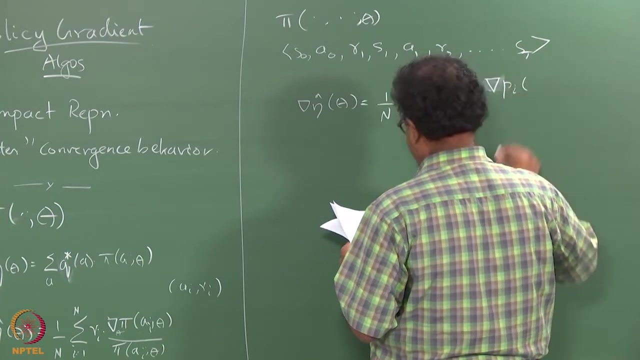 I will be collecting trajectories like this, So now what I can do…. I forgot what notation we use for this. 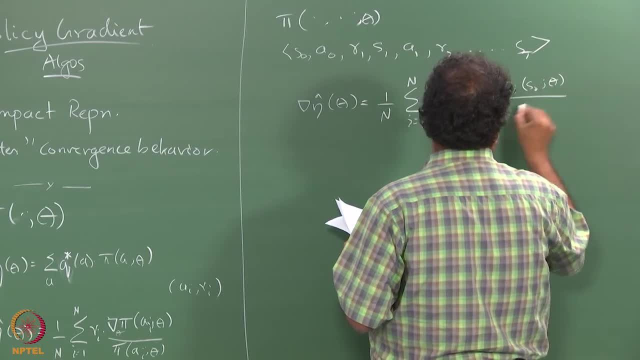 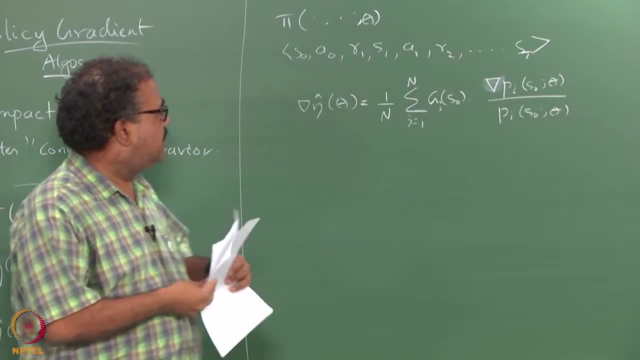 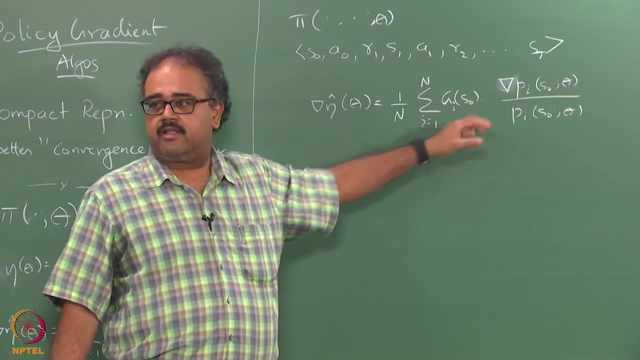 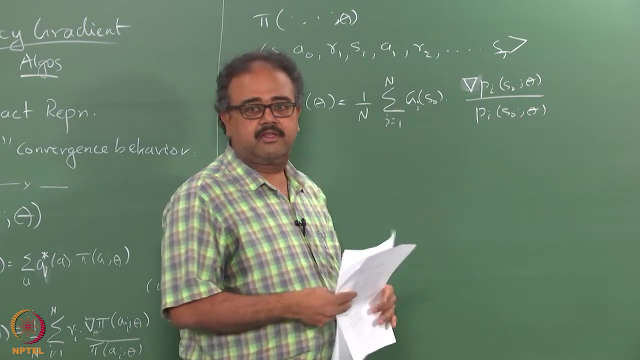 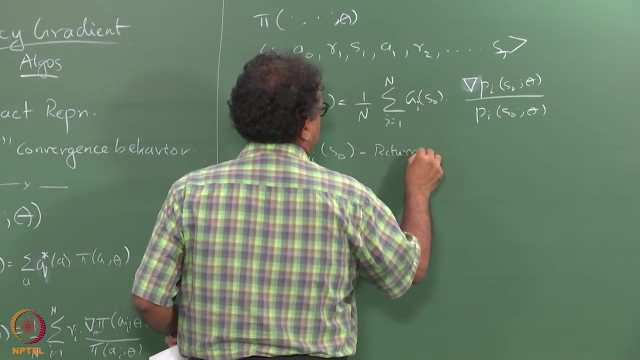 I forgot what notation we use for this, but this is g i, which is the return on the ith sample starting from s naught, and this is the probability of seeing the ith sample starting from s naught. Right, Okay, Okay. 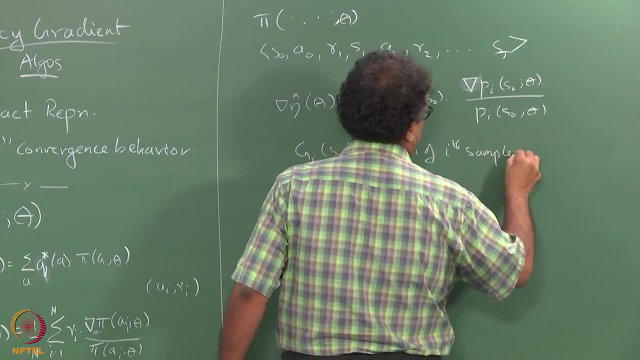 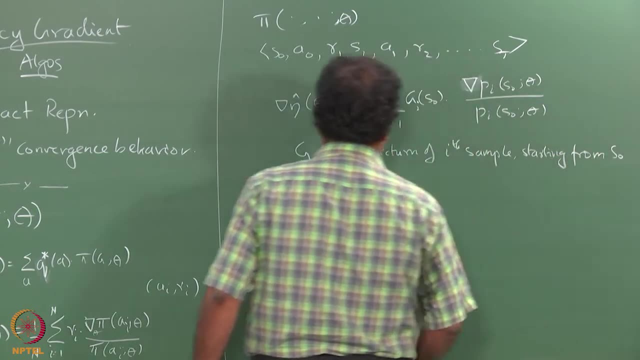 So we can ask for an expression in, say, two values and we can ask for an expression in one value. Okay, So we'll start with g, All right? So g is the distance between the initial values of the second and last diminutive. 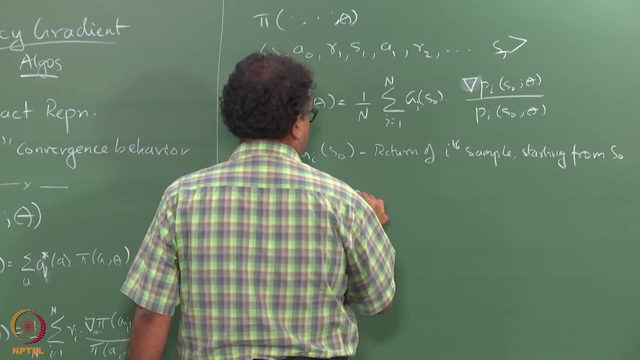 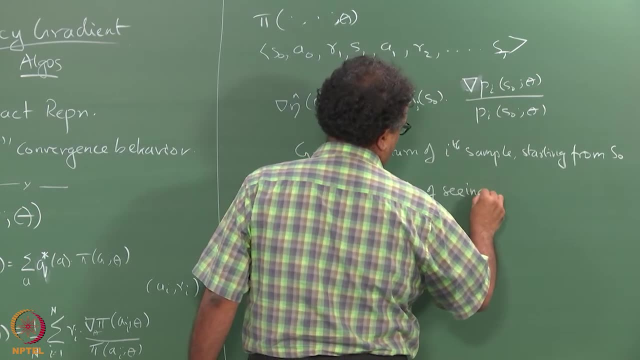 values. Now we can ask for a value right. If you're well aware of this and you want to do an equation of f of one, g is equal to f of one. all right, We can do it like this. 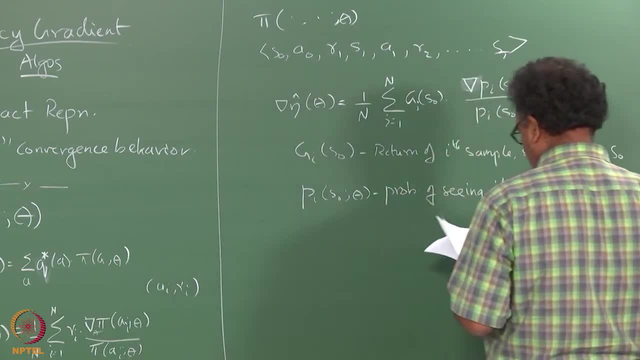 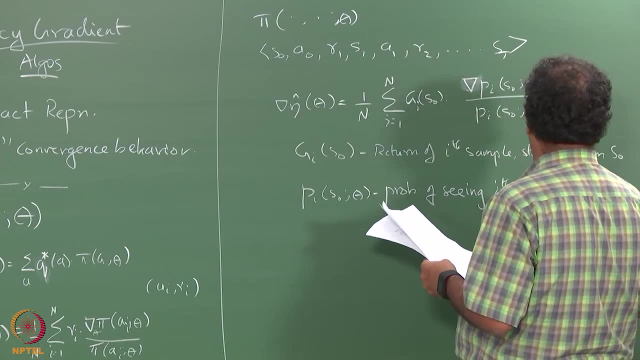 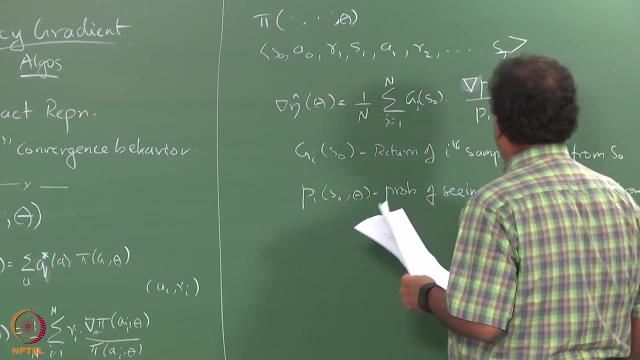 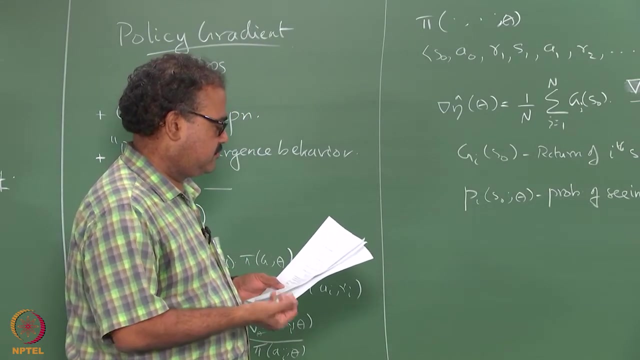 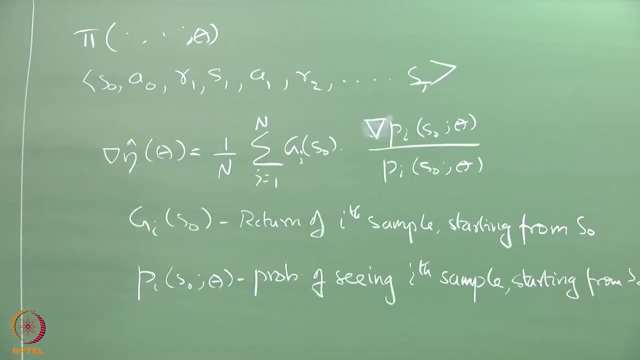 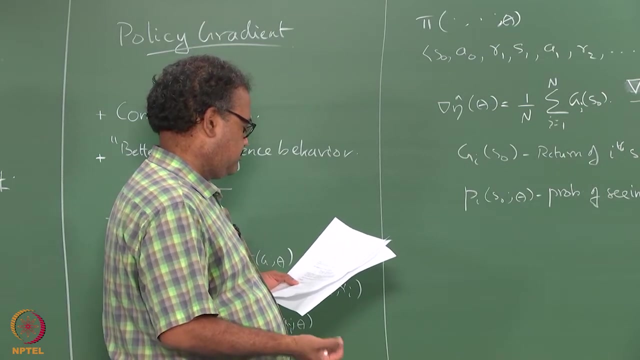 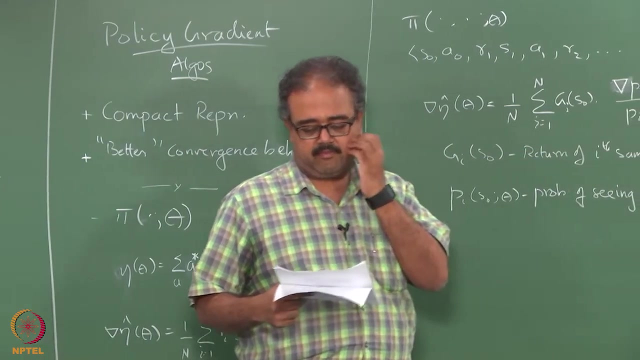 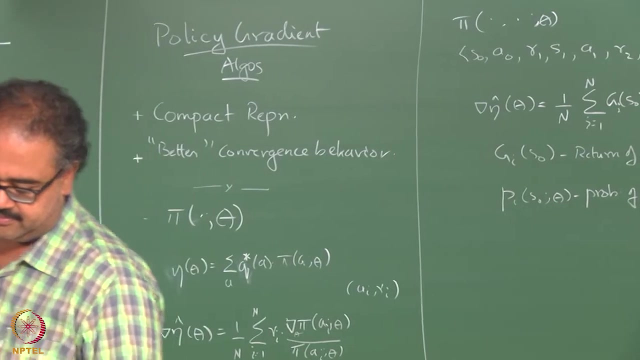 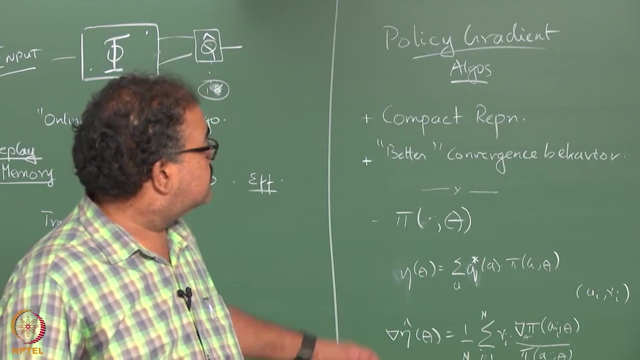 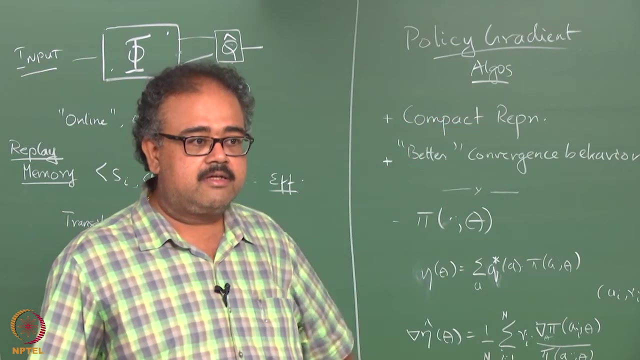 There's a better way, Okay, Okay, We can do a better way than that. All right, Thank you. So what is this probability? P? i The trajectory right That S naught A naught R 1, the whole probability of seeing. that is the probability of the. 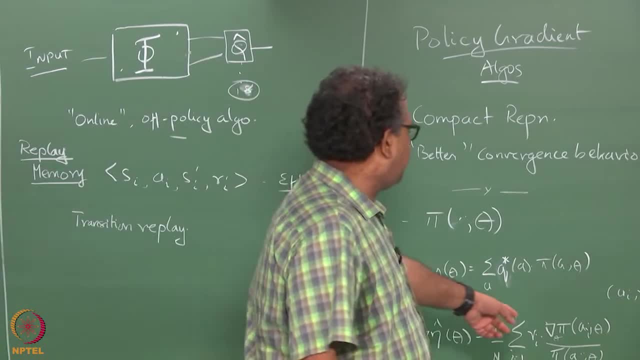 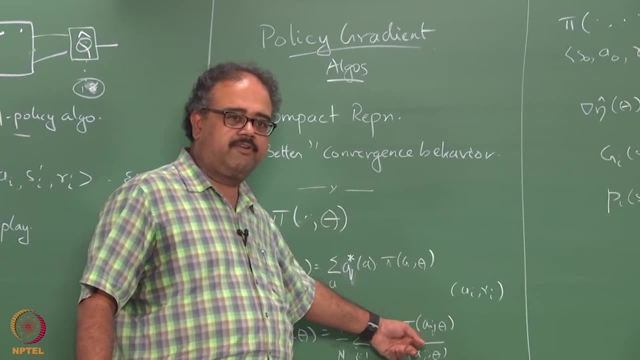 sample. right, Let us see. So what did we do here? We said I take action A i and then I am going to get R i. So this probability of taking action A i is here right, Then I get R i. 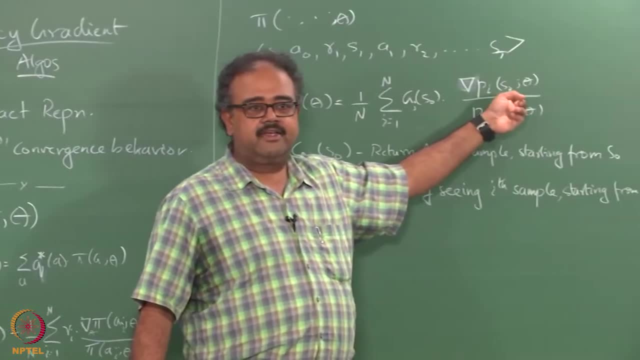 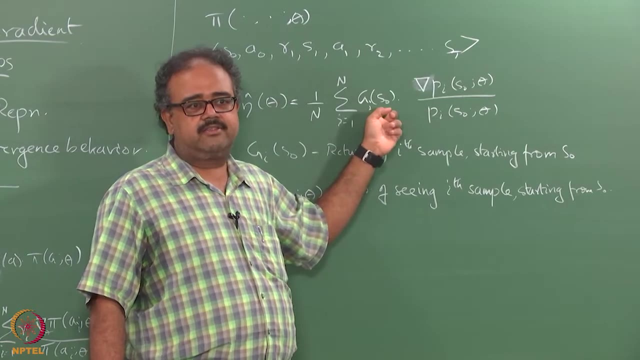 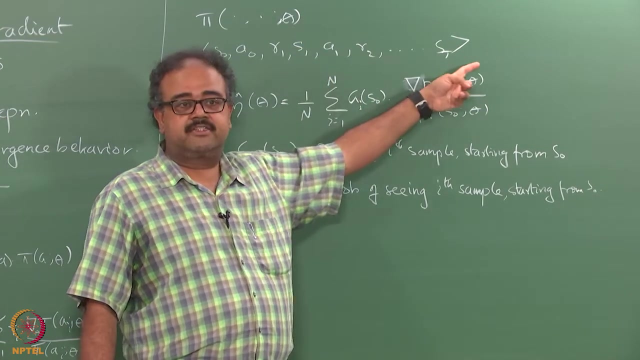 Here. similarly, the probability of taking this trajectory is here. and if I take this trajectory then I get V i. Okay, Okay, Given this trajectory, G i is. probability of G i is 1, because the rewards are all fixed in the trajectory right. 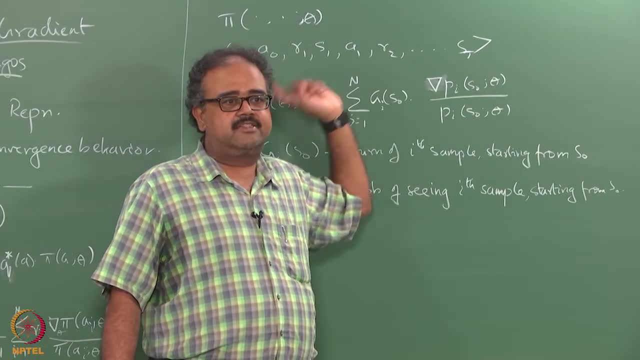 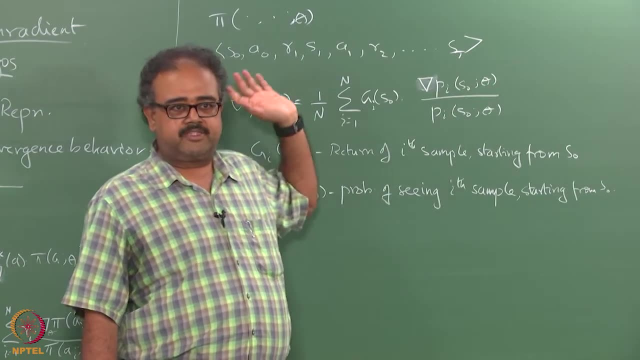 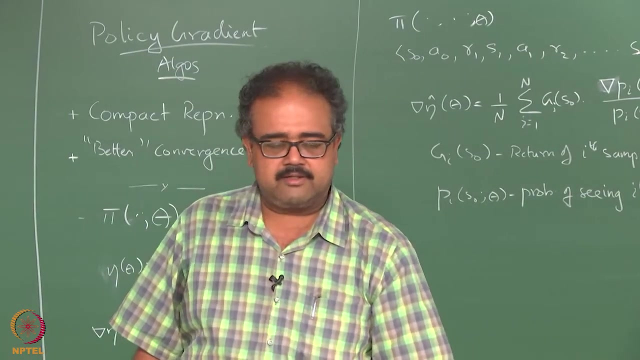 Given this trajectory, the probability of G i is 1,. but what is the likelihood that I will actually take this trajectory Under policy? that is why the theta is here- right Under this policy, pi. what is the probability of me taking this trajectory right? 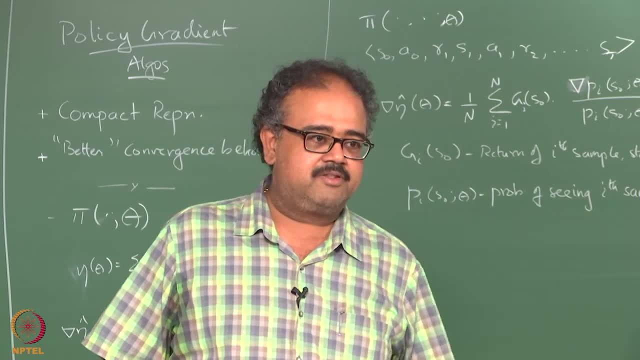 Off policy when we talked about, which are not a policy plus a policy minus one right- The product of policy learning. the product of policy learning when we talked about it is very similar to the off policy learning, Except that there are one policy at the top, one policy at the bottom. 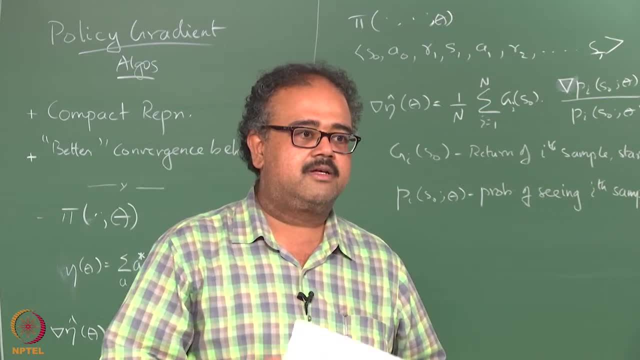 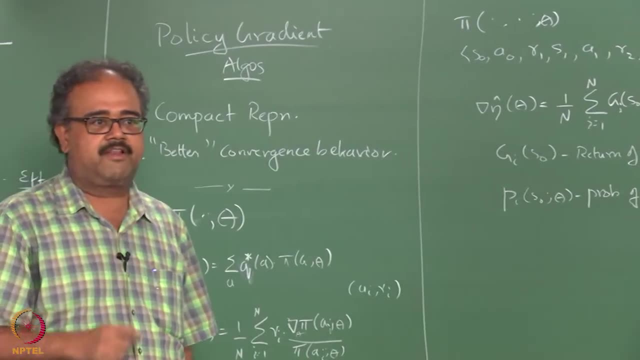 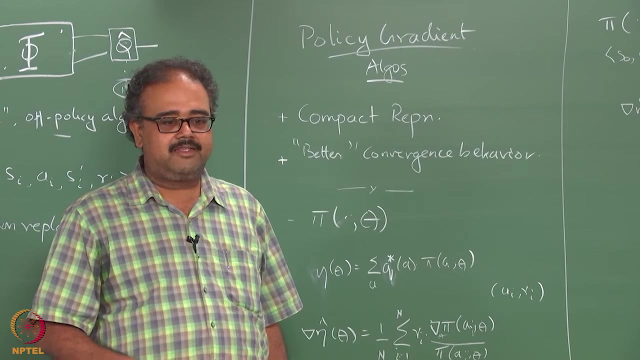 The transition probability is 1, dependent on theta they are going to cancel, but if you do a little bit of sleight of hand, I can actually convert the product. It is a product, right, It is a product. If you think about it, it is actually a product term. 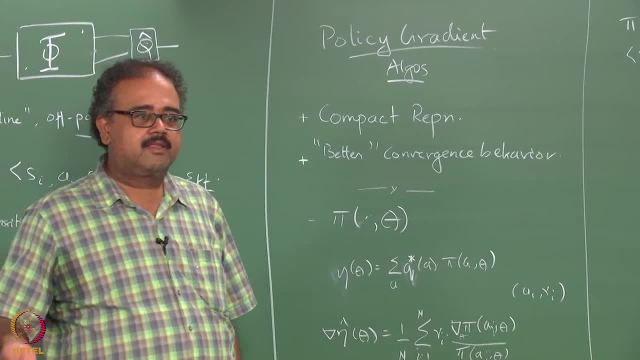 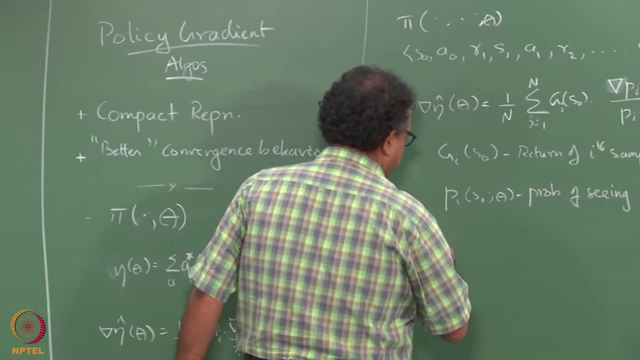 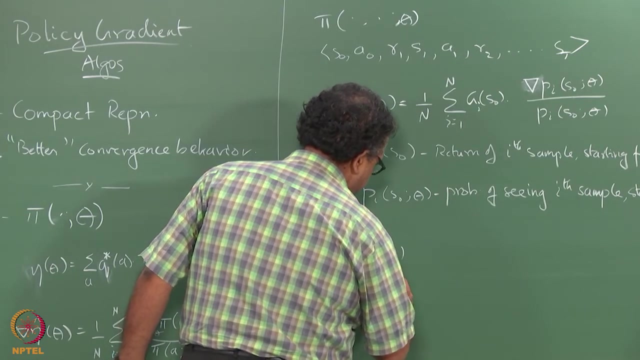 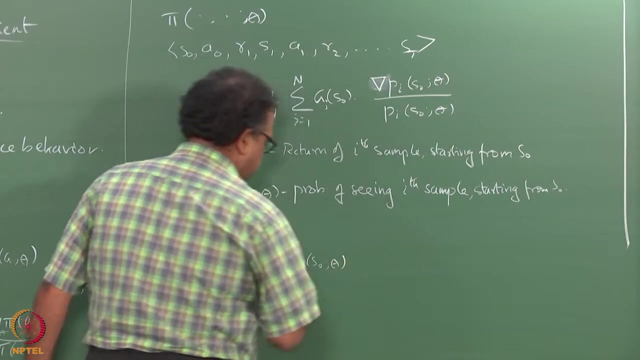 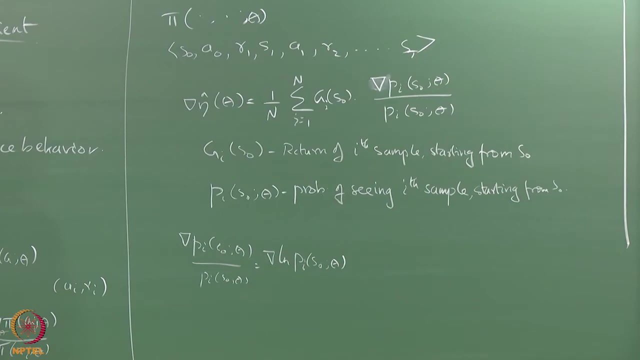 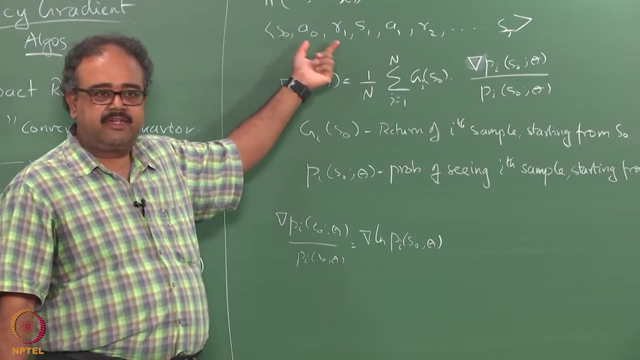 You can convert the product term into some term. It is actually derivative of the log. So this thing, do not try to write pi first and simplify it. take this right. So now, what is pi? Pi is the probability of taking a naught in S times the probability of going to S- 1 times the probability of picking. 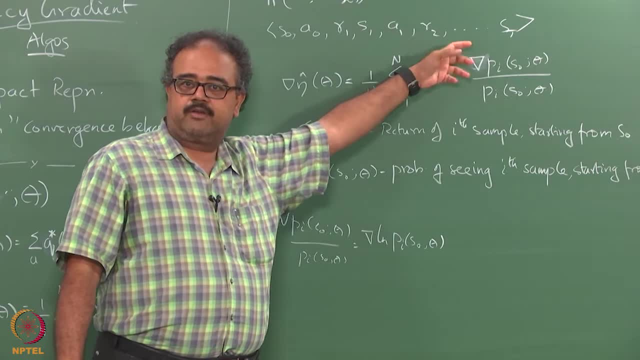 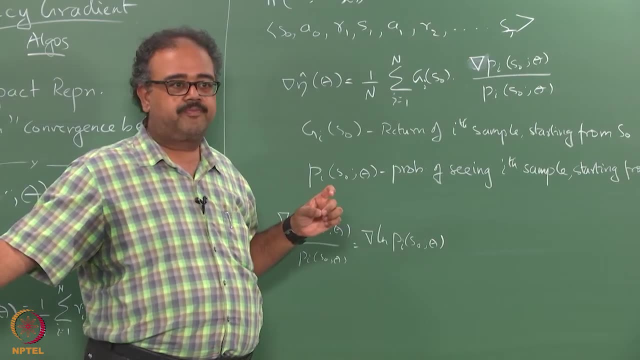 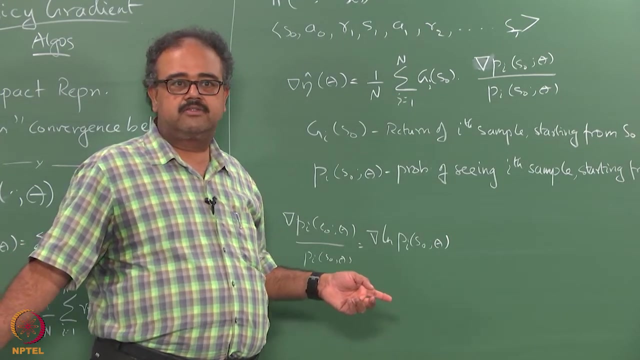 a 1.. 1 in S S: 1 times the probability of going to blah, blah, blah, all of those things. Then times the probability of seeing R 1. given you have picked this, all of this is actually a very long product, So that product can be written as: So it is lawn of the product. 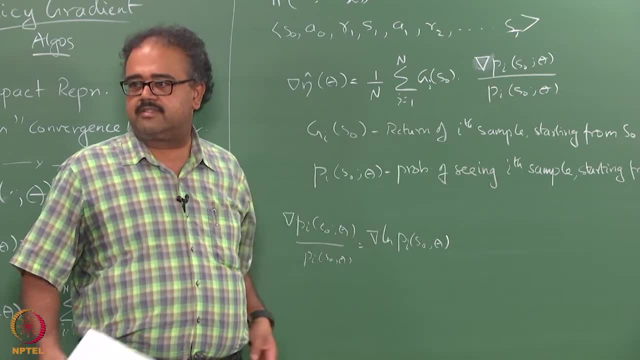 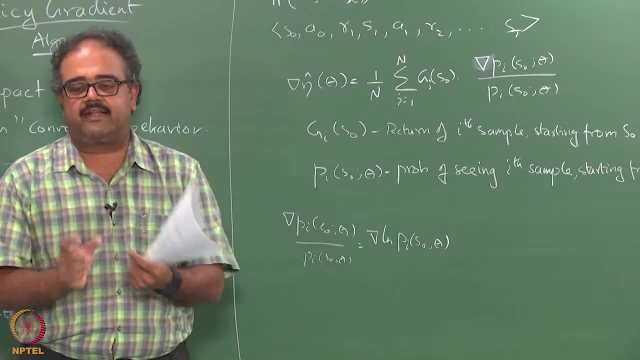 right? So it is some of the lawns, So I can write it as the some of the lawns. So what will be the terms I sum over will be exactly the ones that I want to cancel out, right? So essentially I will say sum of lawn going. 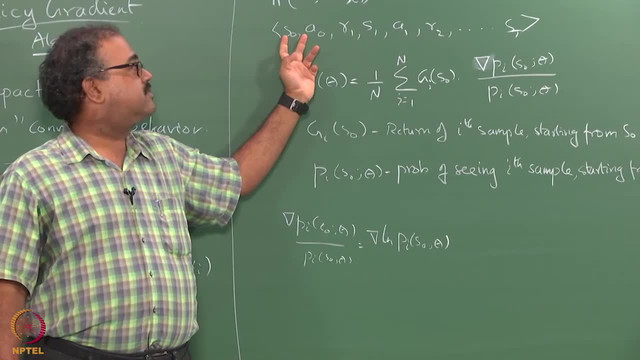 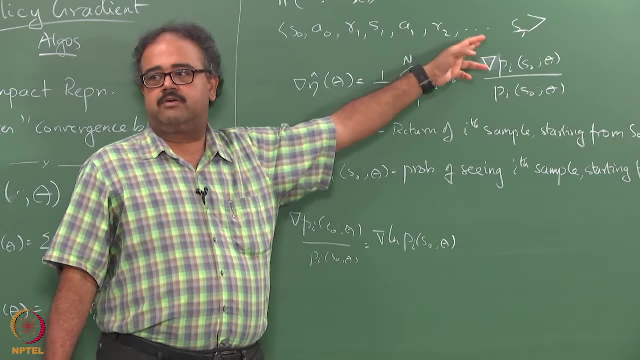 from S naught to given S naught. A naught going to S 1 times the probability of going from S 1 A 1 to S 2.. So all of that if you take as one term, they will all cancel out because 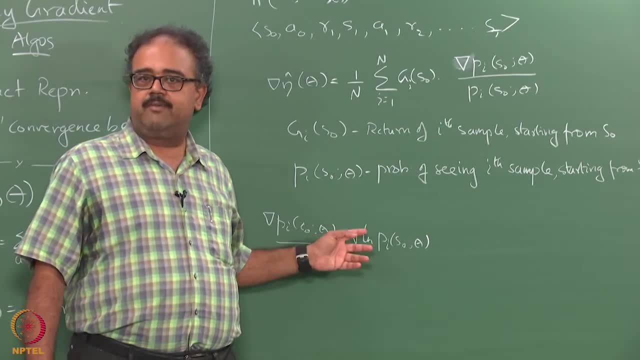 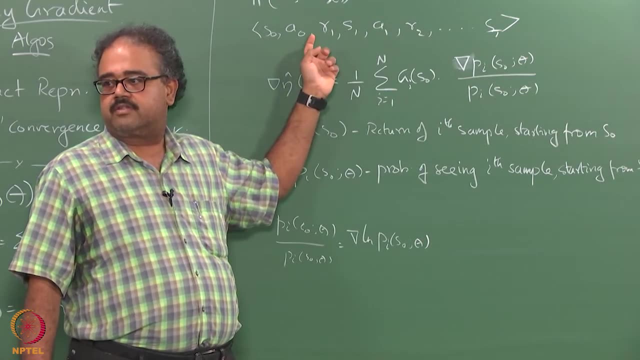 the derivative will be 0, right? So what will be left out, with the probability of taking action A naught in S naught and the probability of taking action A 1 in S 1 and so on, so forth. So that will, those will be the only terms. I will be left out, right? So this essentially. 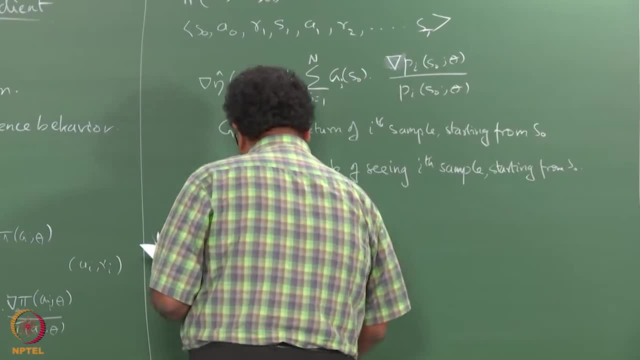 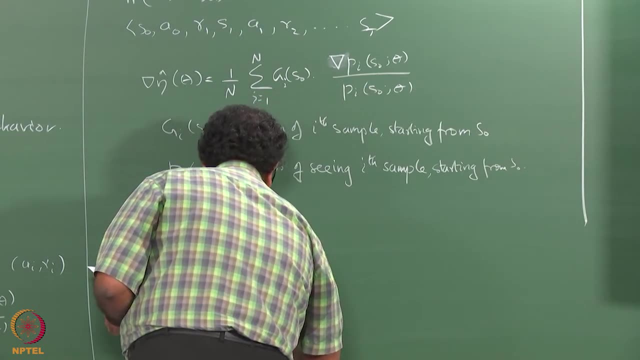 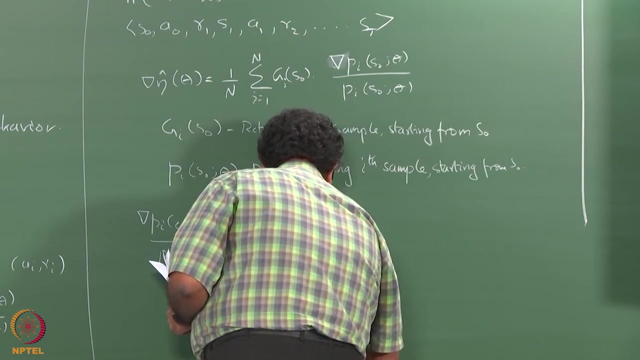 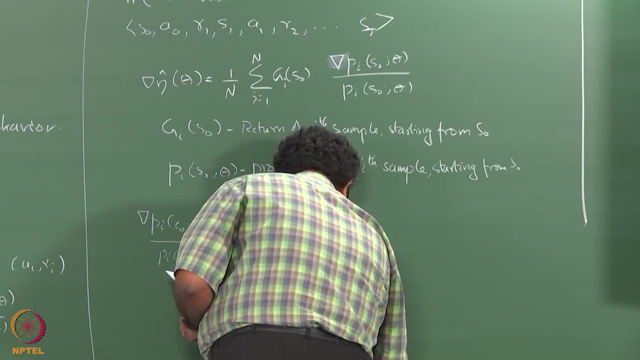 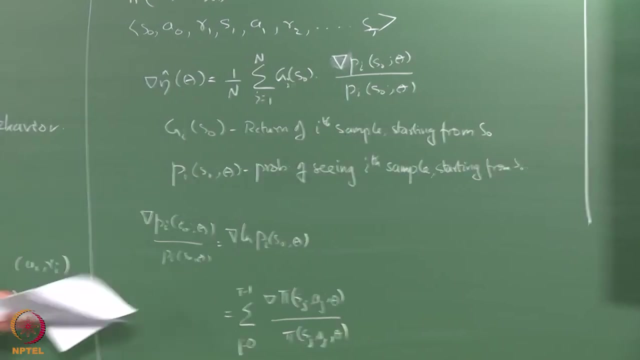 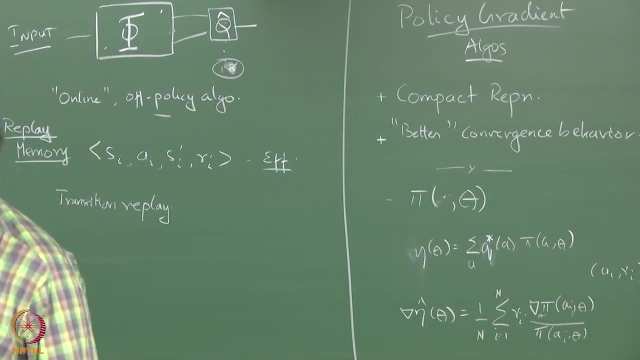 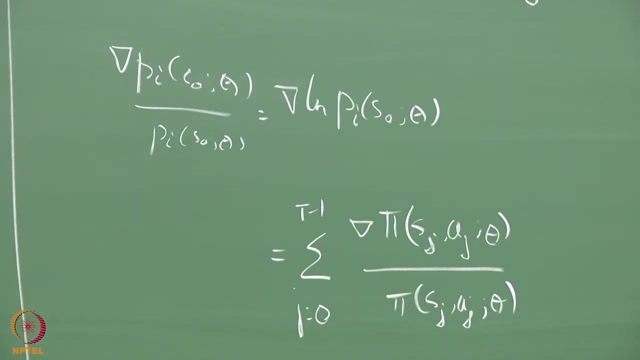 reduces to. I am not going to work it out, you can do that. 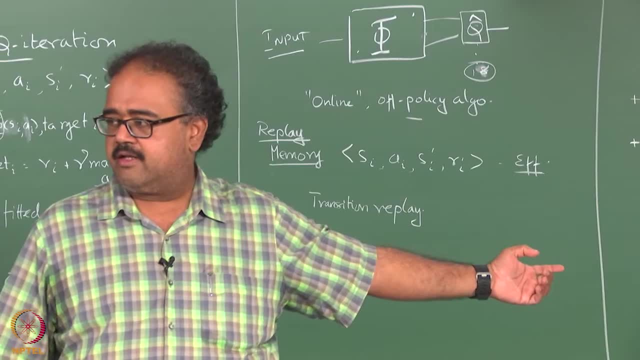 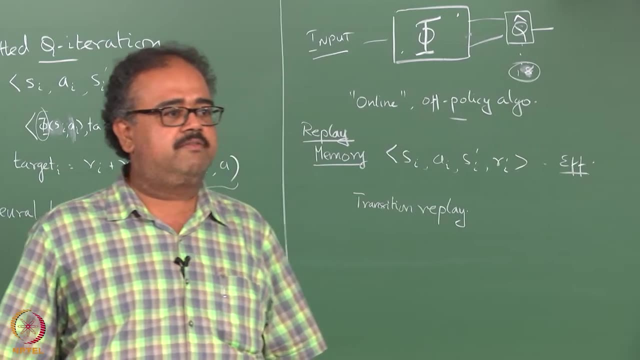 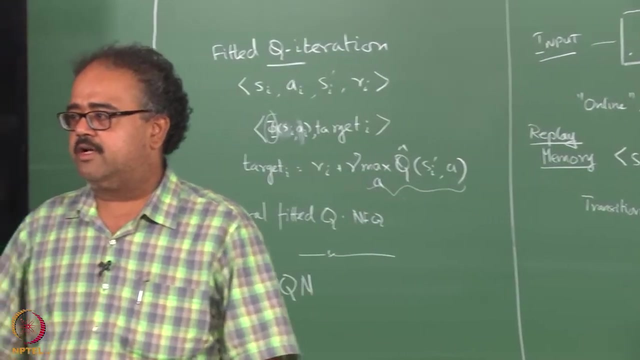 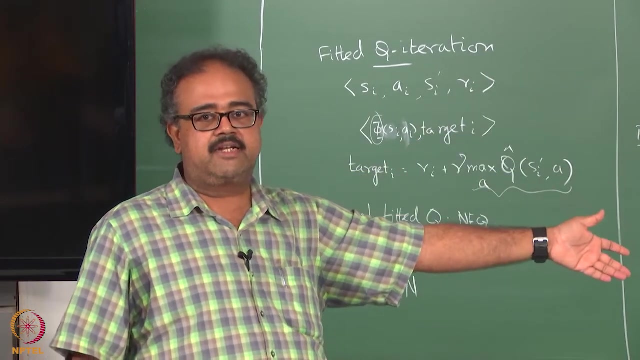 right and see which of those will where the gradient will vanish right. and then, whatever is the left out terms, are the exactly the ones that I have written that right. so, even though I do not know p? i, because I do not know the transition probability, I can write: 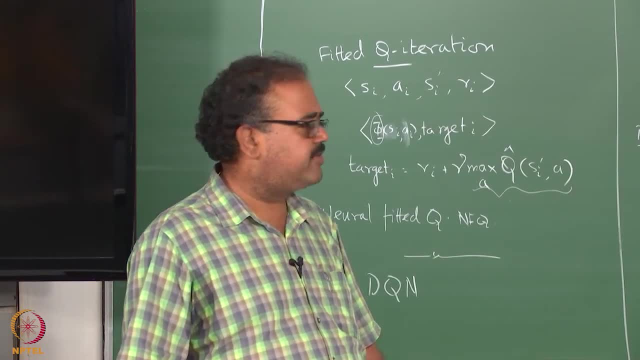 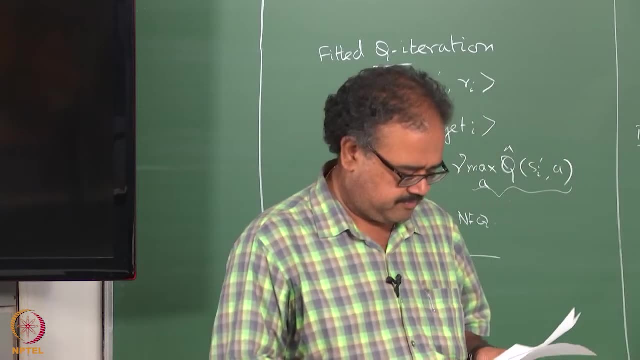 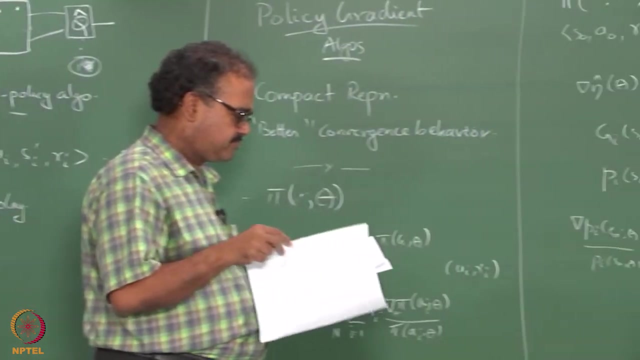 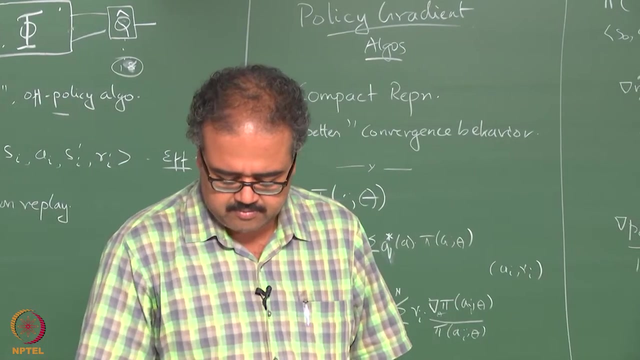 the ratio or the. this is called the likelihood ratio. if you remember, I can write the likelihood ratio as just the terms in pi. there is one small thing which I have kind of any any questions on this. so once I estimate the gradient then I can essentially update. 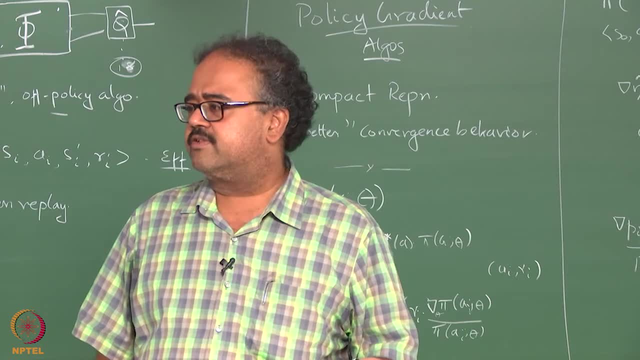 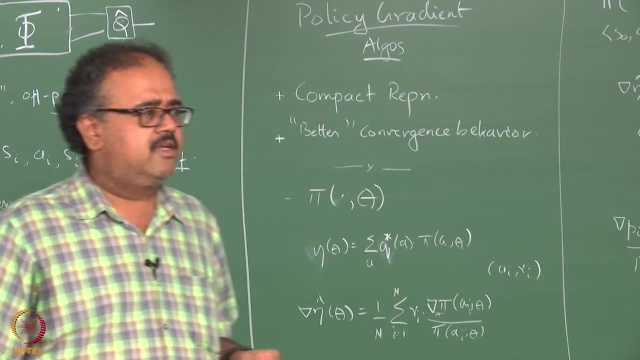 my parameters along the direction of the gradient right. I can do an online update, I can do increment and incremental update. whatever I want to do, I can do, I can. we have various variants of whether I am doing online, incremental, so on, so forth, but that is one thing which I 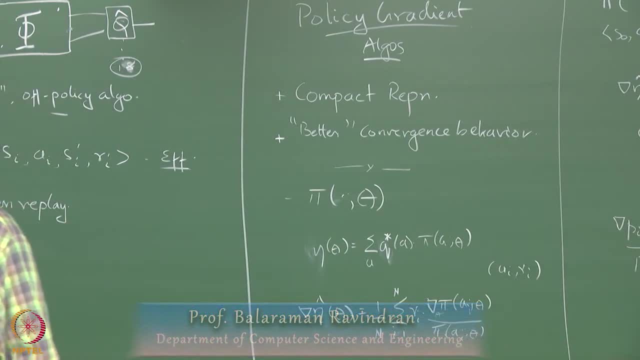 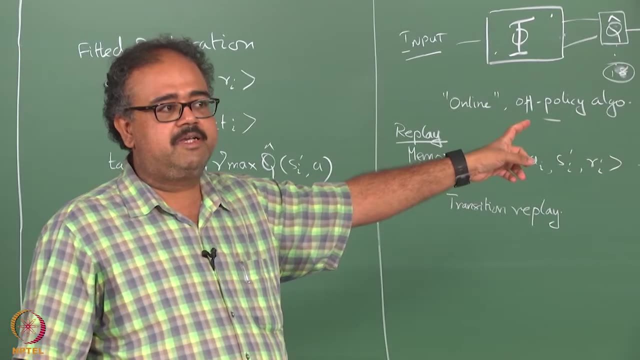 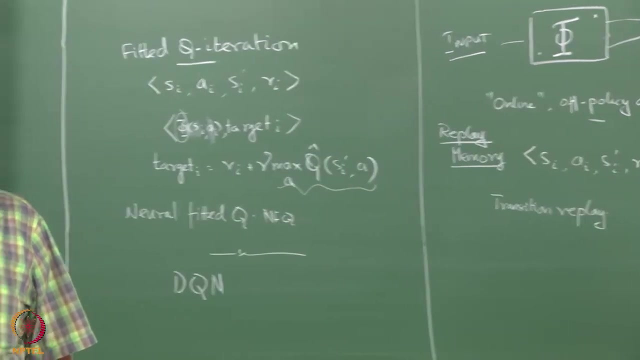 have done a small slight here. right, explicitly talk about it. if you look at the performance measure, eta, right, the performance measure may depends, it is a function of theta alone. right, it does not depend on state s or anything like that, right? so essentially here there is no notion of a value function associated with the state, but I still need a notion of 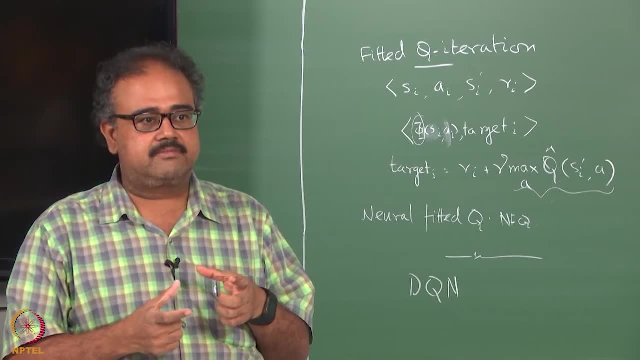 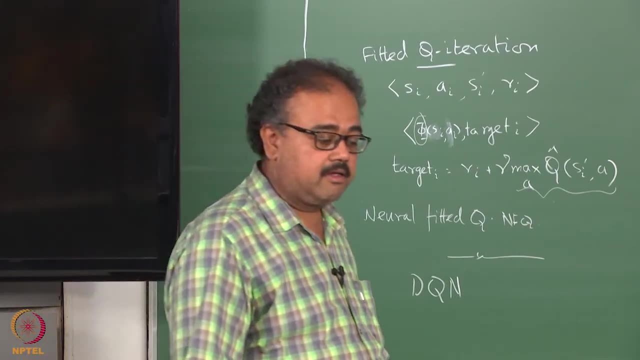 a value function associated with the state, but I still need a notion of a value function associated with the state. but I still need a notion of a value function that summarizes the utility of a policy right. and what I have I done here? no, what have I done to give a single value for the policy right. I mean, if you remember, 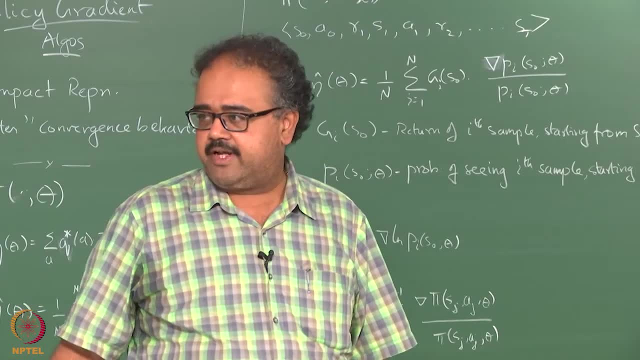 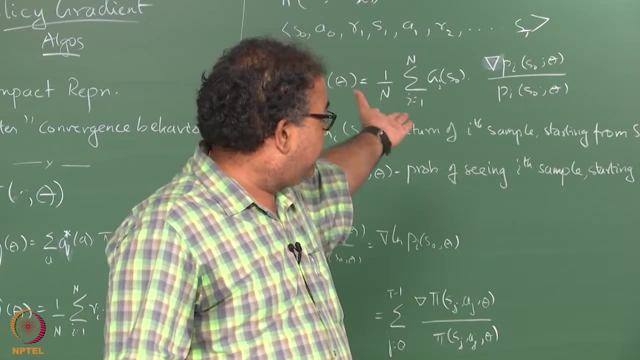 the value function case. for every starting in every state, I have a different value, right? but now I am saying I will use a single value for the entire policy. so how did I get that single value for the entire policy? what have I done here? okay, yes, all right. 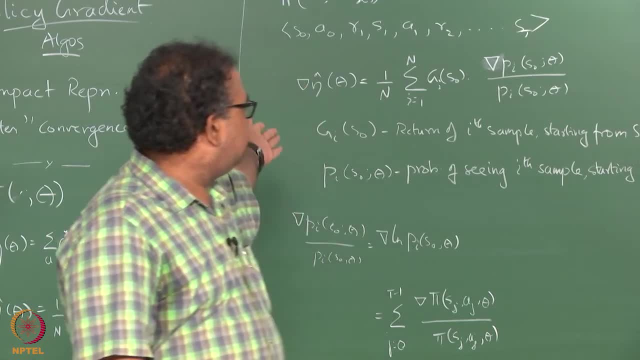 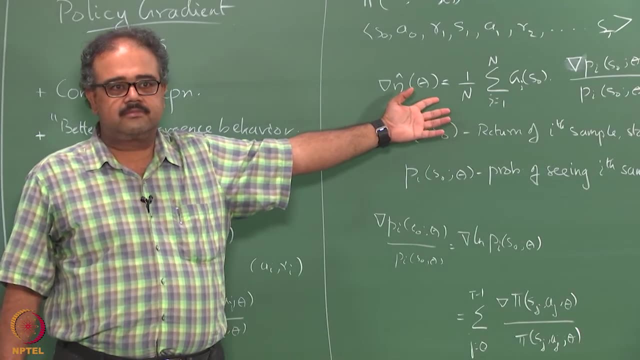 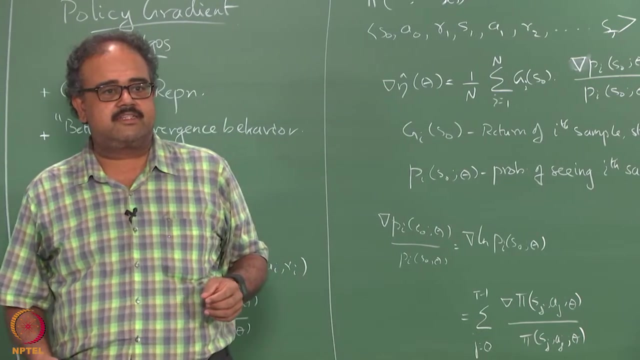 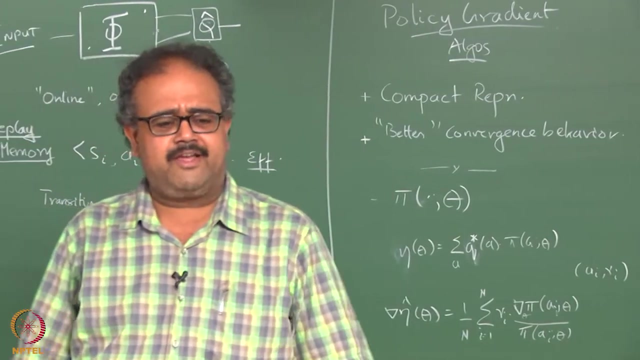 The s naught does not have an i on it. I am assuming there is a unique start state, right? I am assuming there is a unique start state and I am using the returns from that unique start states as the evaluation for the policy right. this is fine right if you think about. 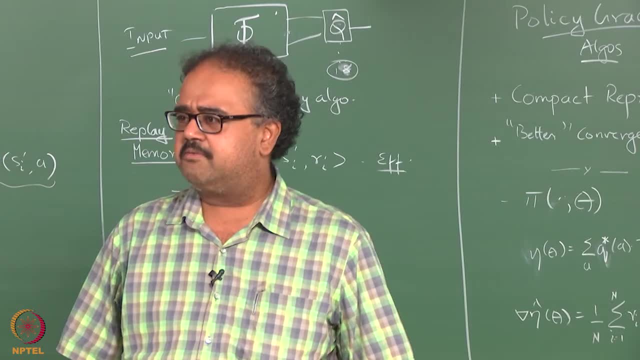 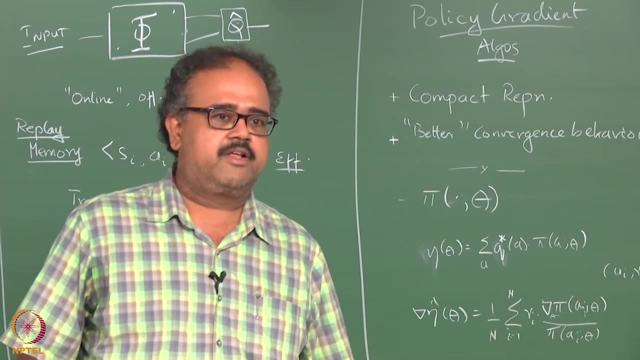 board games right. always you will start at the same board game right, lot of other control things. you will always start at some particular given a certain amount of resources and you always start in a particular start configuration and so on, so forth, right. so in many cases, 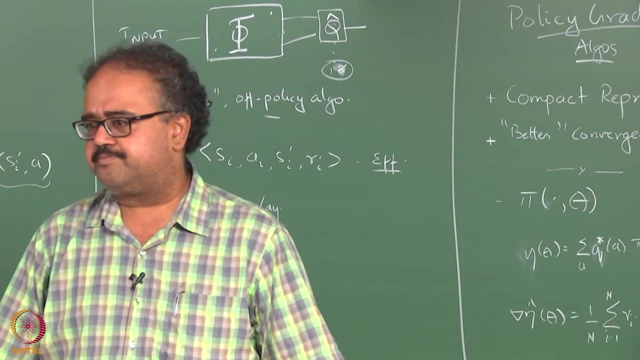 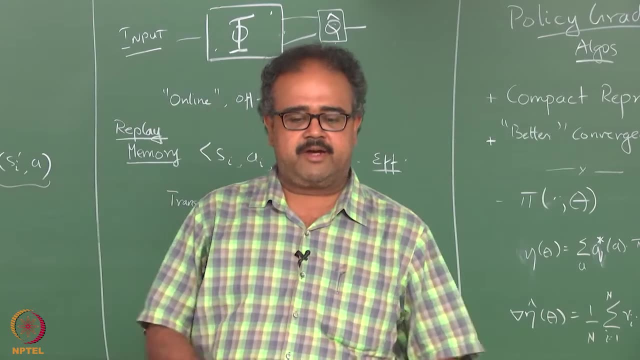 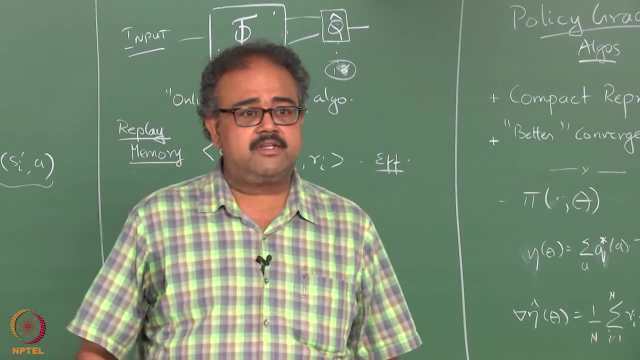 this is actually an acceptable thing to do, right using a unique start state. What happens if you have, instead of a single start state, but you have a set of states over which you can start? you can take an imaginary start state and with uniform probability. 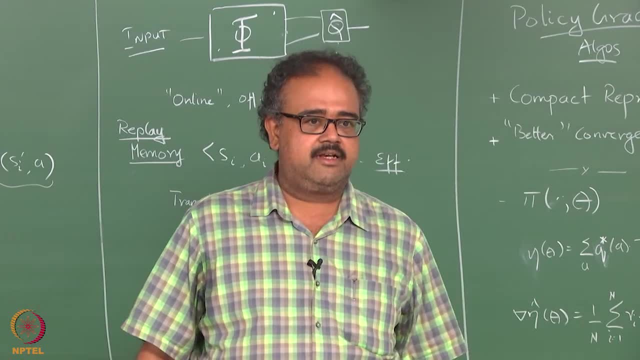 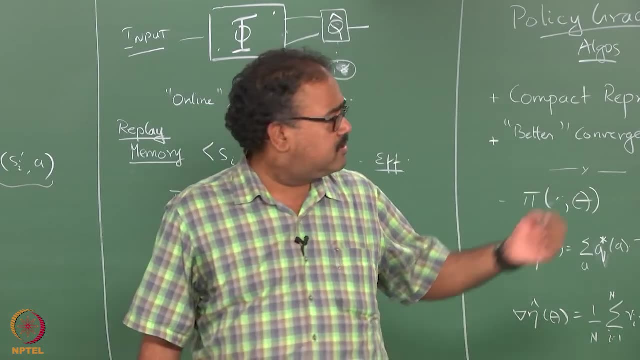 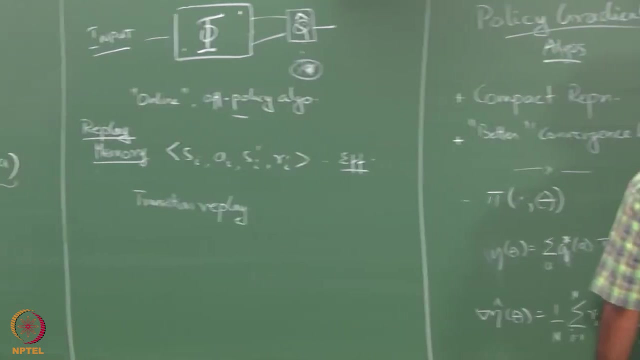 you can transition to one of those states So without any action, and from there you run your trajectory. so then you look at the value of this imaginary. so we spoke about this earlier also, right, So with? so I am basically using this s naught as my unique, as a unique start state, right? 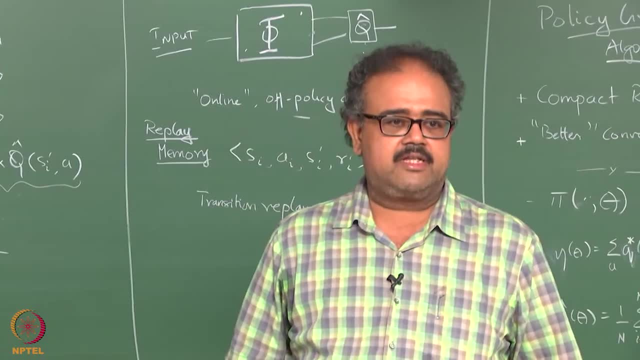 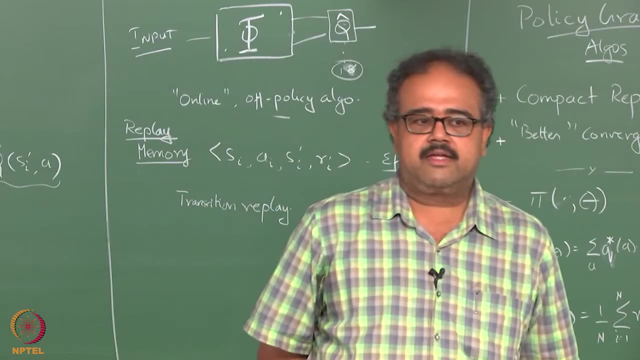 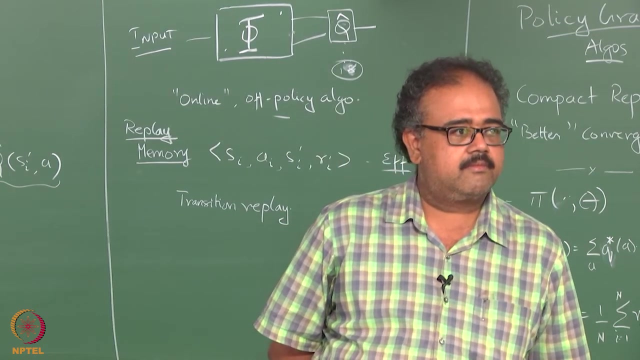 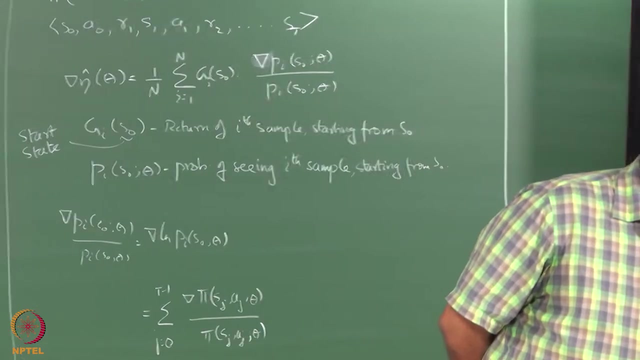 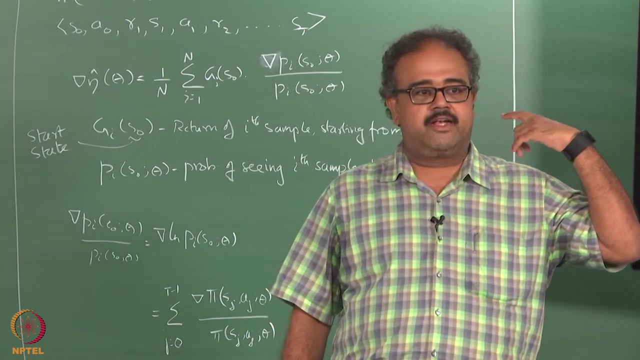 but more commonly, there is another, another assumption that we make for reducing into a single value function, single value for a policy. So what is the assumption we make? yeah, I mean, as with all Monte Carlo methods, that you need to assume that the trajectory ends here. right, if your trajectory is running on. 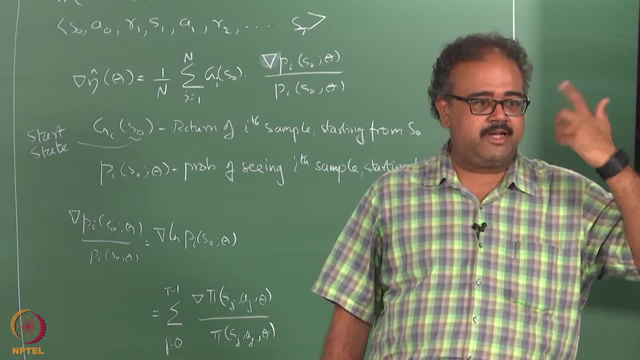 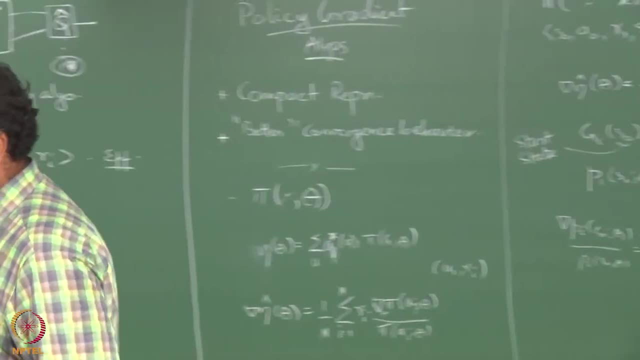 forever. you cannot use this method as it is. you will. you will need to modify it somehow. I will. I will talk about that in a bit. but that is not the end state, is not the issue here. So there is something else which people do, which is exactly where the average reward. 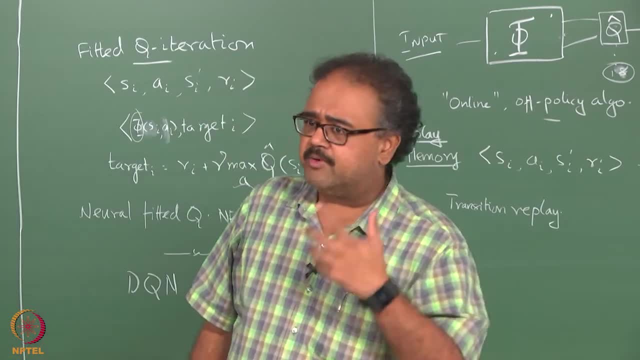 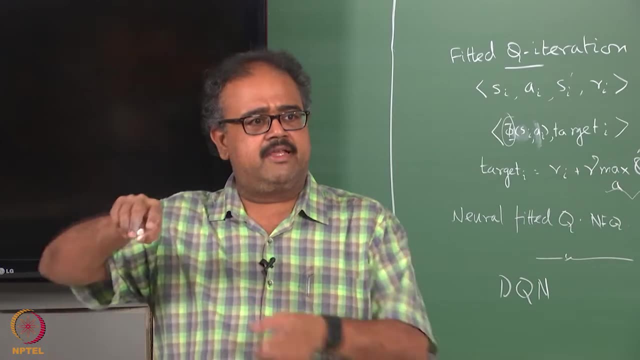 R L will fit in right. So, if you think about it, what does average reward reinforcement learning tell you? right, we already looked at the average reward formulation, right? So 1 by n, as n tends to infinity. R 1, 2, right? So R 1, R 1, R, 2, R 3 plus R n, right? So, essentially, 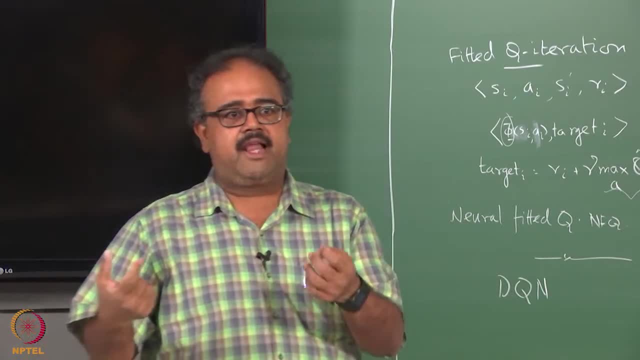 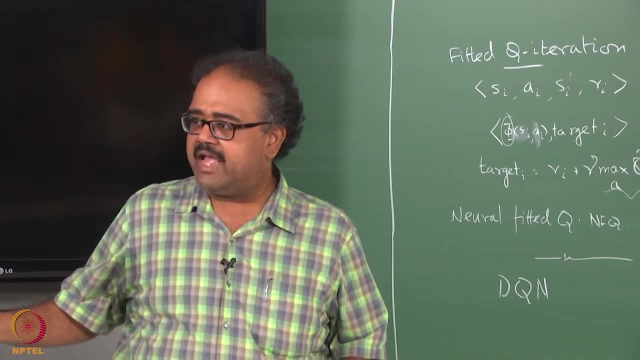 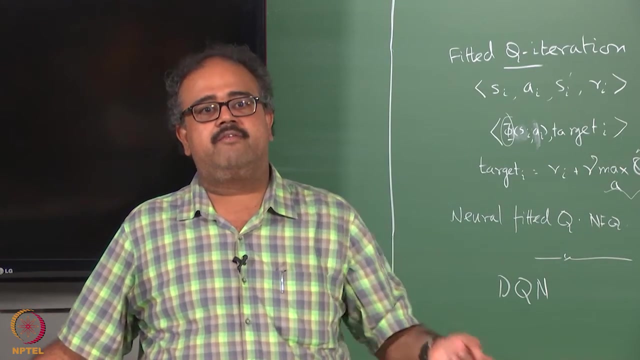 you take the average over n steps and then, as n tends to infinity, you compute them right right. So, if you think about it, because n tends to infinity, any initial variations that you would see in the value for starting in state 1 versus starting in state 2 will all get. 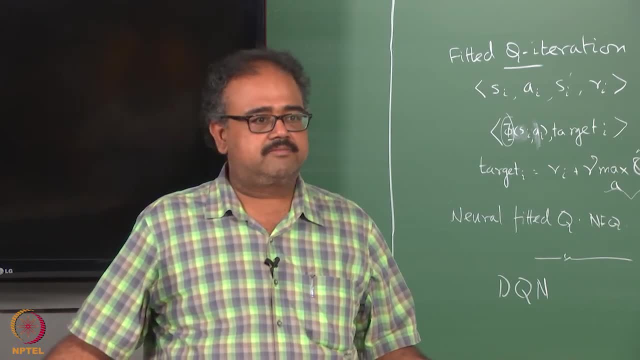 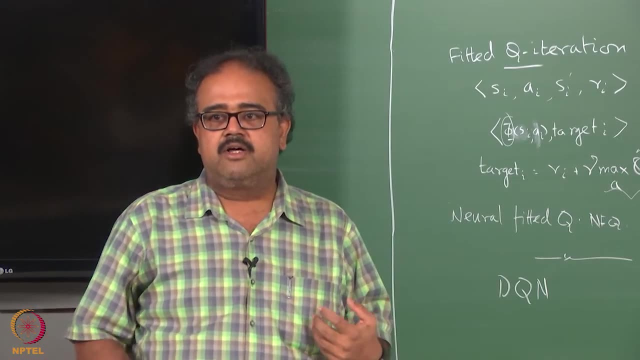 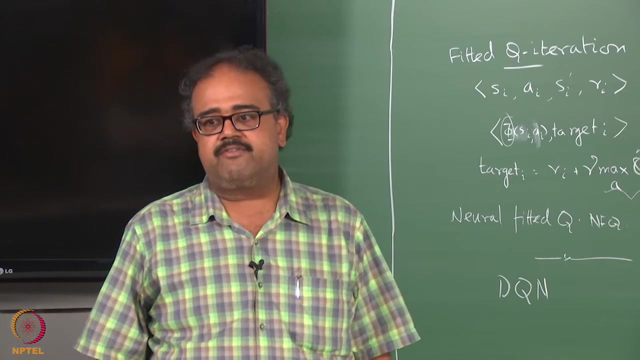 wiped out. right? Any initial variations will get wiped out because you are summing up a infinite number of infinite series of numbers. So as n tends to infinity, the values for starting from any state will. average value for a policy starting from any state will. 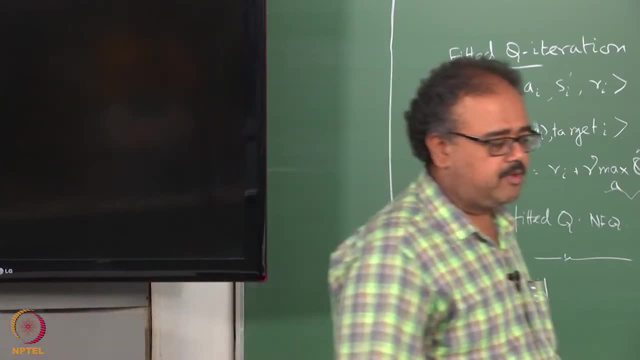 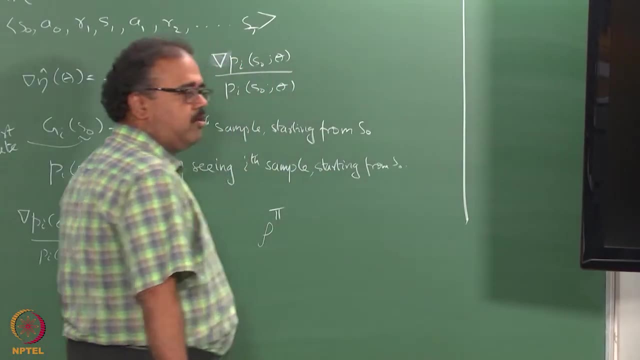 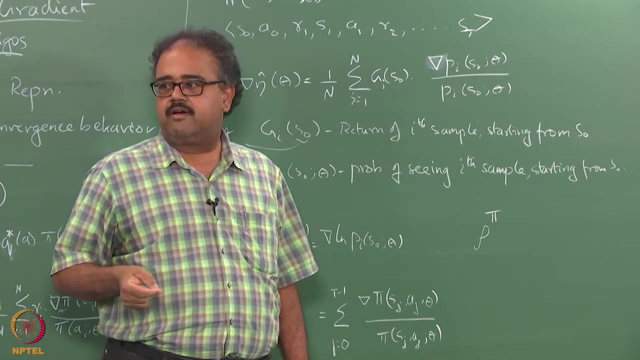 be same quantity. So in average rewards, right, So you, essentially, you have only something called rho pi, right It is no, it is like we value function v, we have. So in average reward, you have value of a policy denoted by rho pi. okay, regardless of what. 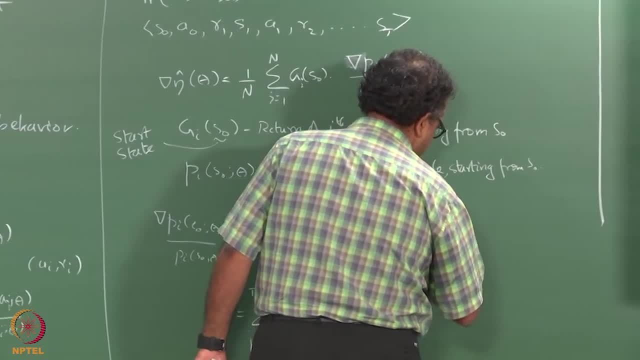 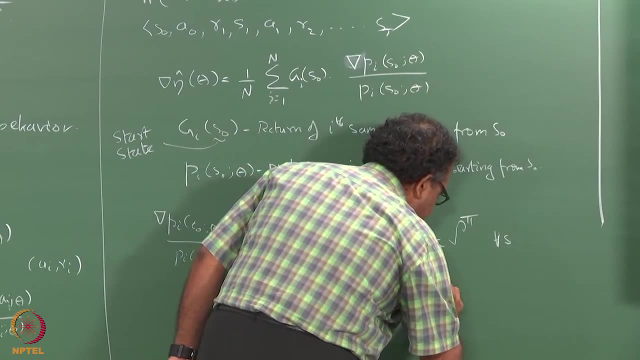 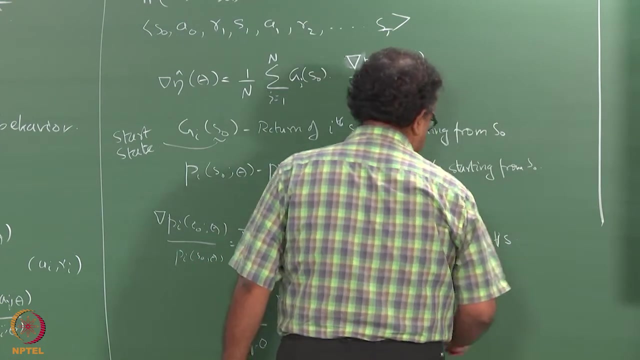 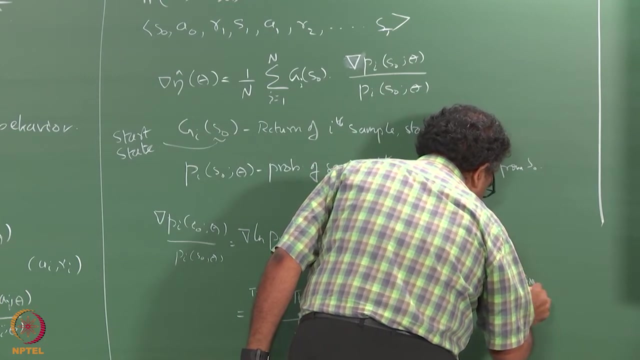 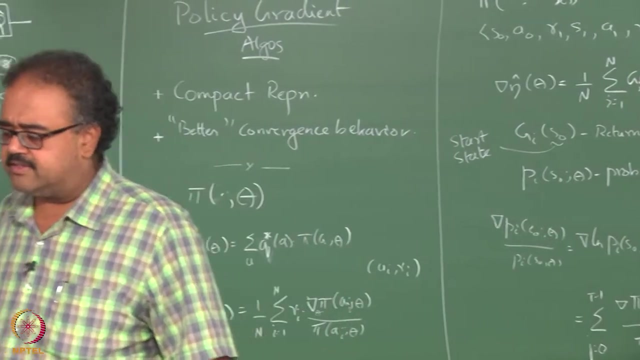 is the state right. So rho pi of s will declare as being equal to the constant rho pi for all s. So you can take the value of rho pi right n that is defined, as of course there are some conditions for all of this average values to exist and be well defined, and so on. so 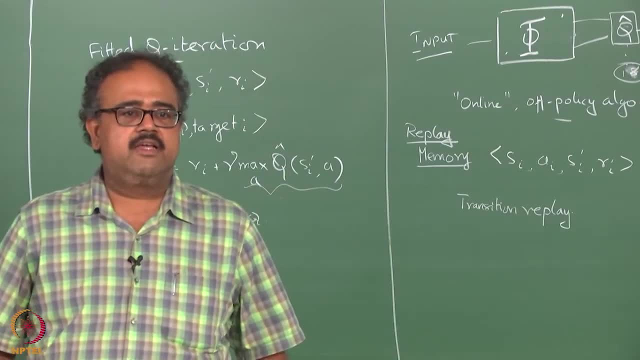 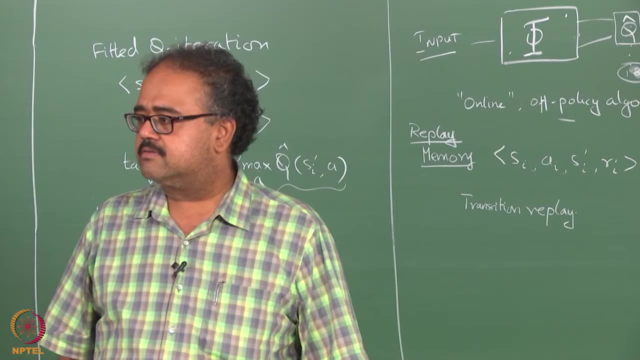 forth. So we are assuming that your m d p satisfies all those conditions, then all we need to do, So it is different, So this is n over n right. So here this is a constant policy: estimate, rho pi, and use that where instead of g i s naught, instead of g i s. 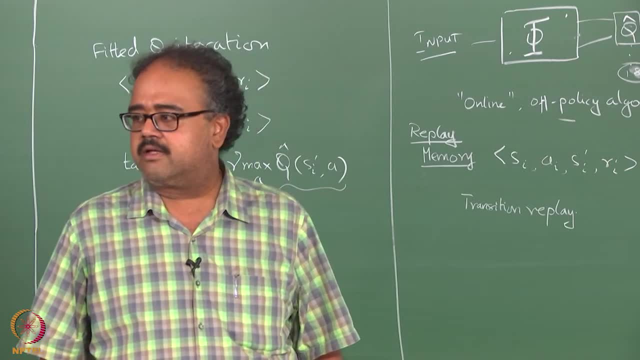 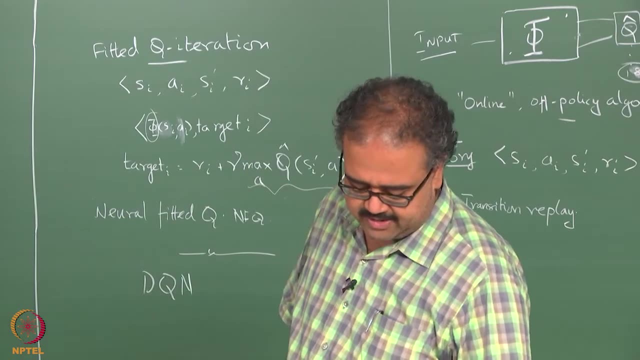 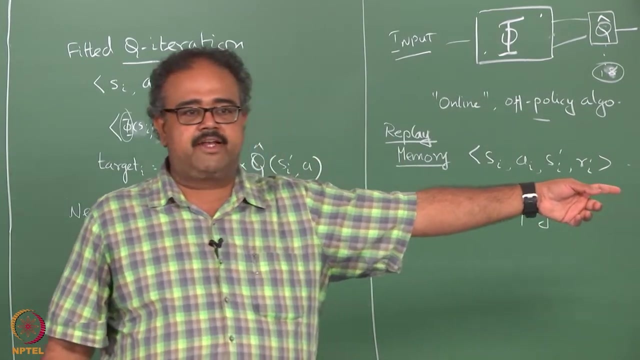 naught, you would use rho pi which, by doing what the average reward will essentially? yes, lower variance thing, right. but the point is well, obviously you are not running until n tends to infinity right? so it is only a sample, right? so it is a sample estimate. 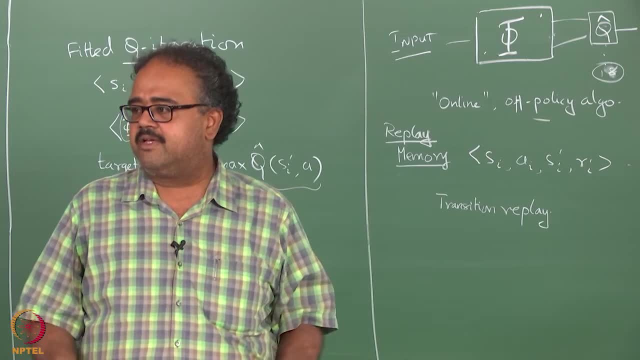 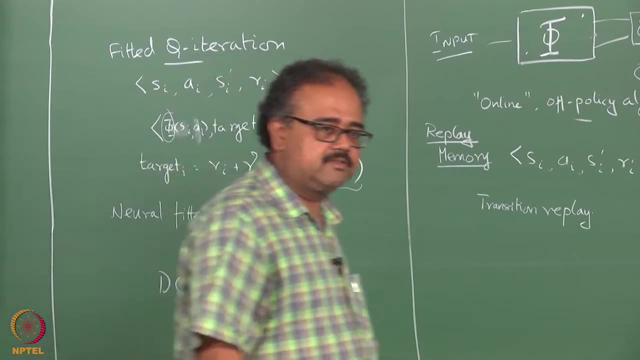 so the rho pi that I use there will not be the same. it is supposed to be the same, but obviously it will not be the same, just like we know that g i s naught will not be the same right. so rho pi is the expected value of this right, so I should put the expectation. 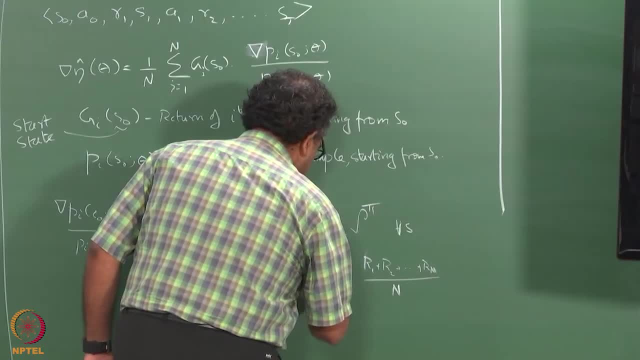 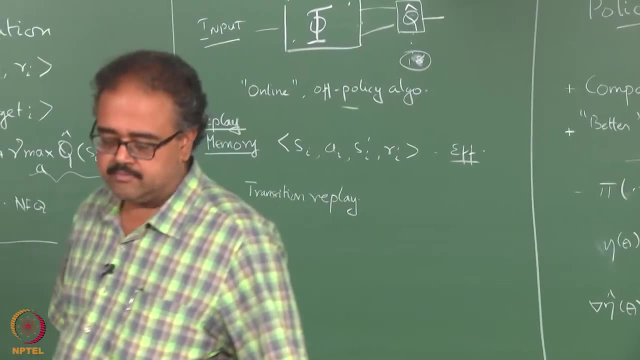 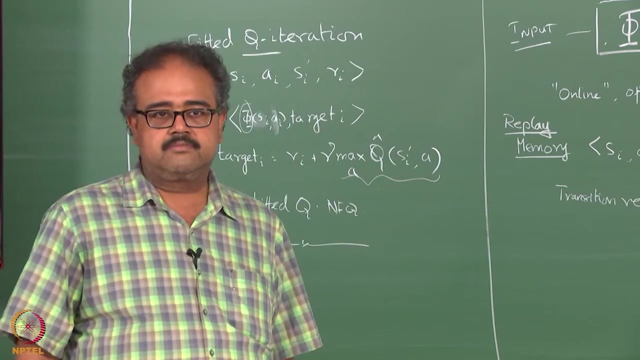 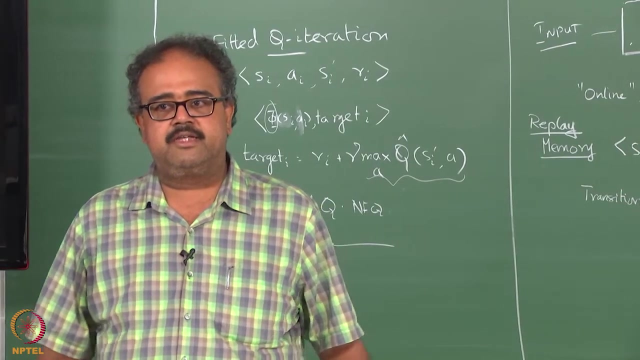 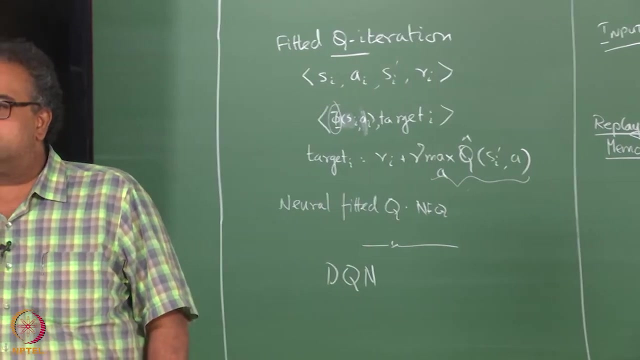 around this right, So I am not going to get into all the nitty-gritties of this. if I have a lecture, I will go do this. I typically do average reward RL, but almost always I find that 90 percent of the 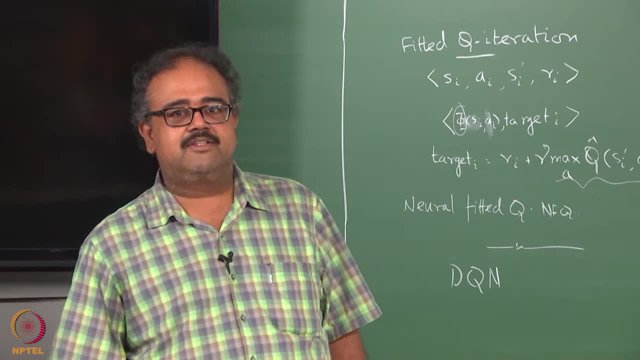 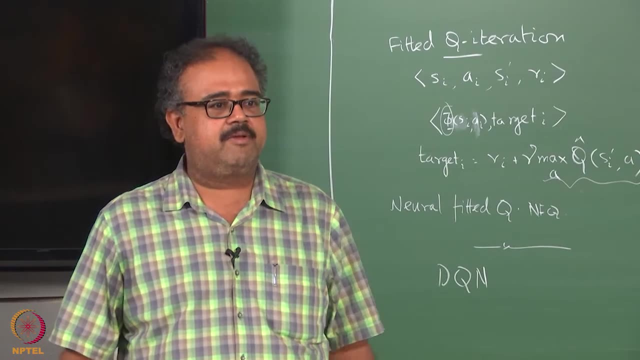 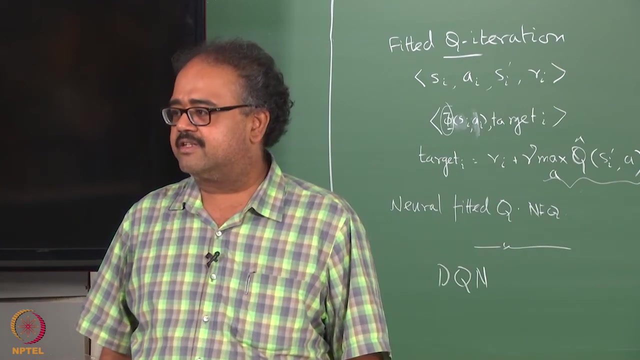 class does not get it. so one lecture is too short a time for me to explain all the nuances of average reward, RL, right. So I end up teaching the class but people not actually getting anything from it. so if you remember that, that is enough for the purposes of this lecture and may be for actor. 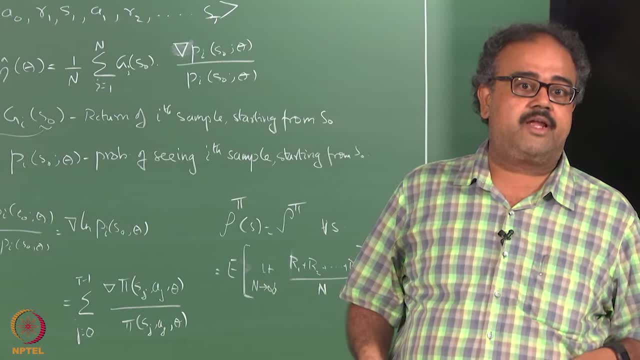 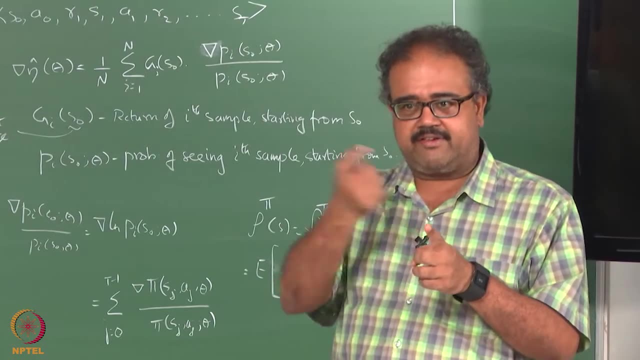 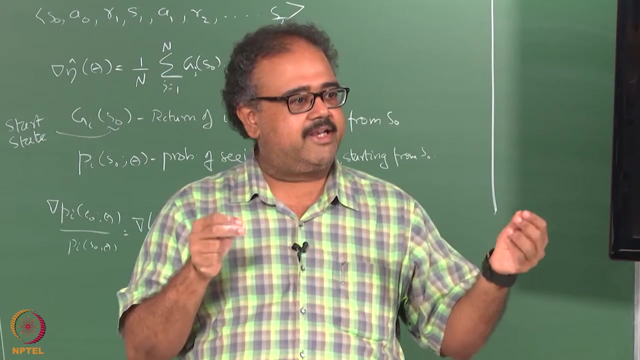 reward. why is it okay to truncate it? See, if I have done enough circles around the states, right, I would have a good enough estimate of the average reward, right? so I do not have to keep doing this infinitely long for me to get an estimate. suppose I go five times around a loop, right, I will. 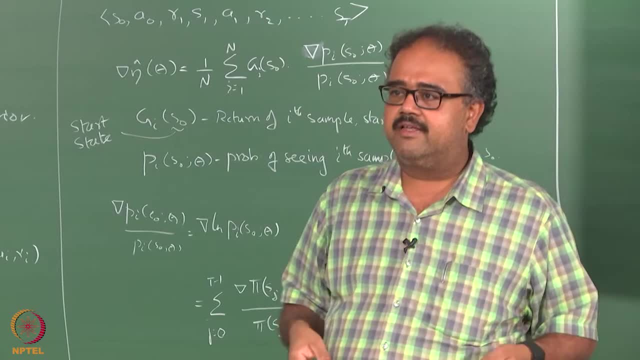 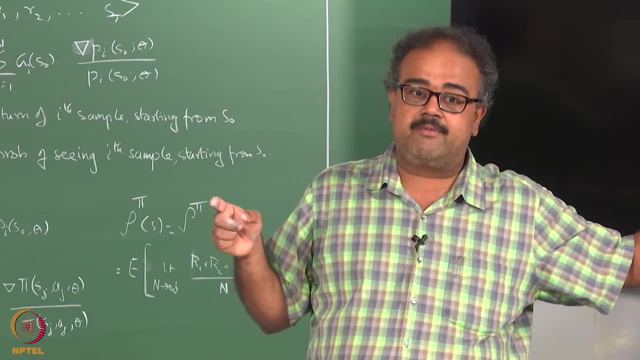 know what is average reward for that loop is right. So sign of roughly Right: so I can do that. so I can, instead of saying that I will run till time, end of time, which might not happen, if I am assuming a recurrent class, it might not end at all. I. 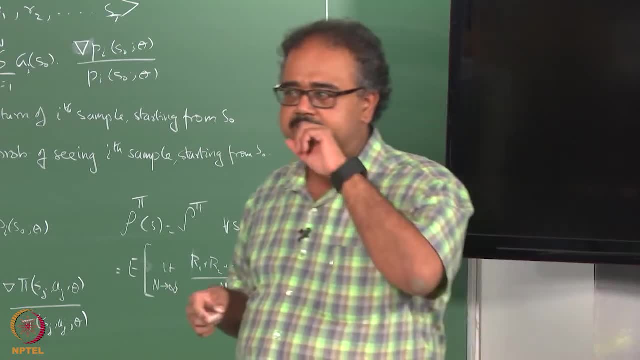 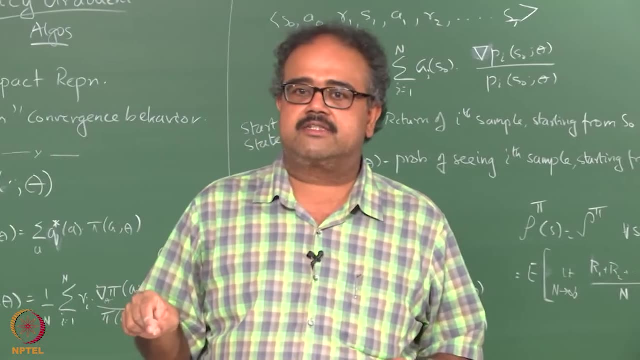 need to have some way of stopping the trajectories. so what typically we do is we say that here is a unique state and stop the trajectory from the state. whenever I reenter the state, I will stop the trajectory. So that is all. I take a bit of the trajectory. I keep doing this, so this will allow me to. 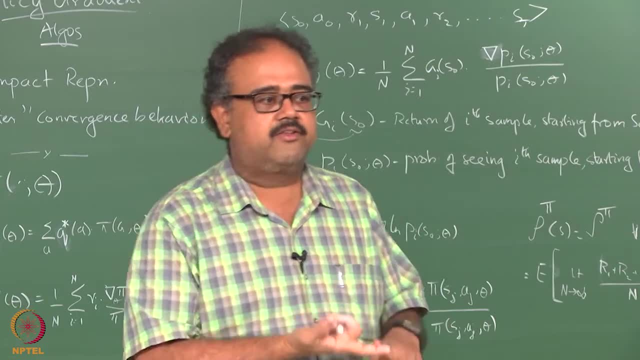 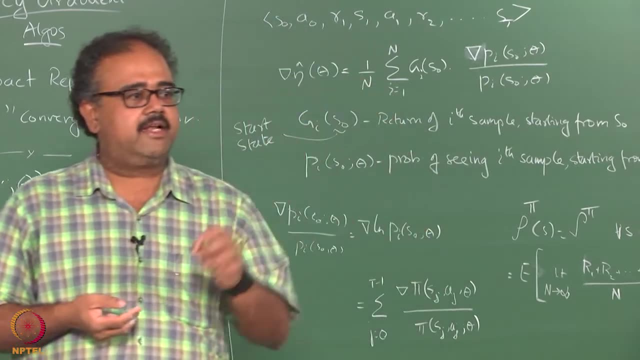 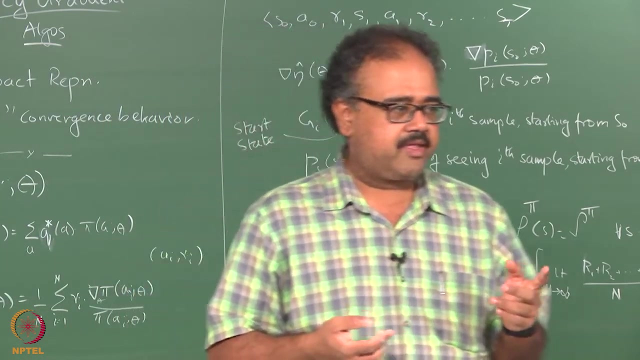 reduce the variation variance. so discounting is one thing. right, so I can. because of discounting, my trajectory will get truncated. the other one is to say that I will designate a unique recurrent state. whenever I enter the recurrent state, I will stop the trajectory even after doing that. 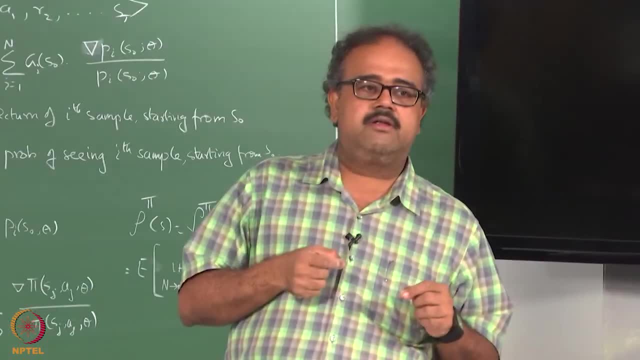 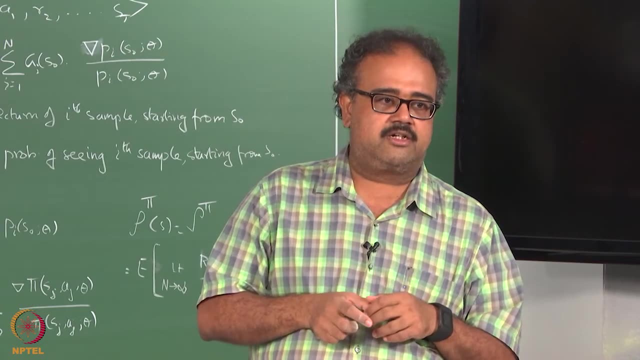 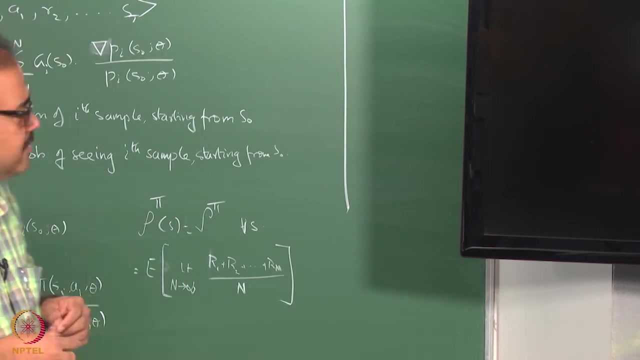 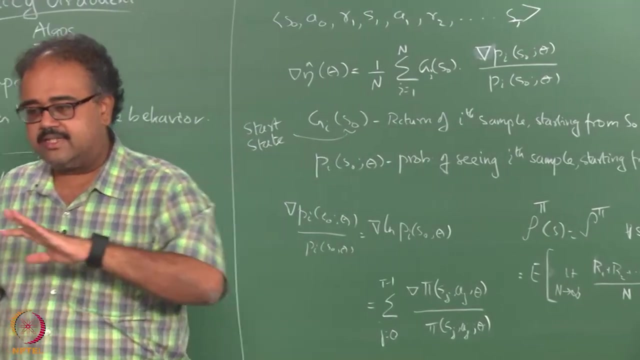 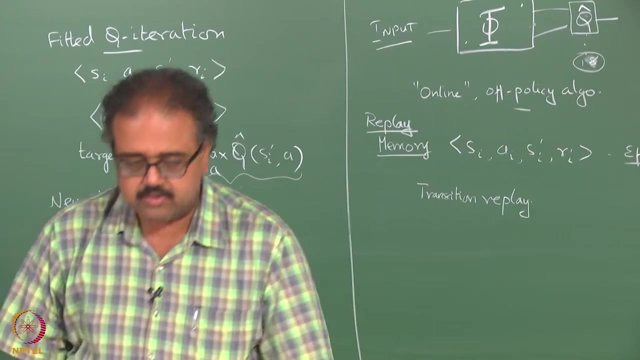 if you get long trajectories, what you can do, you can designate multiple states at which you will stop the trajectories. essentially, the idea is to get shorter and shorter trajectories. So there is another method for reducing variance. so where is the variance coming from? because 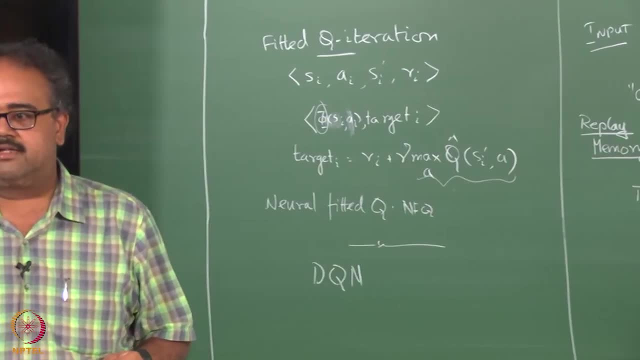 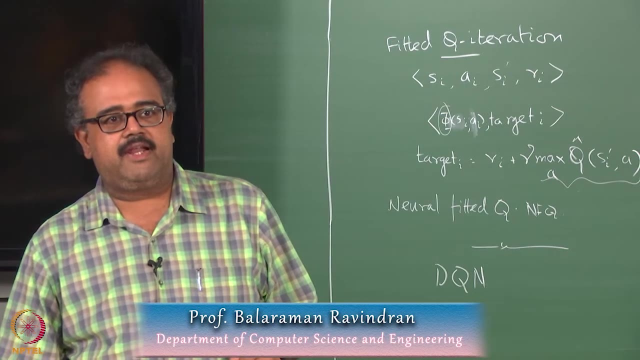 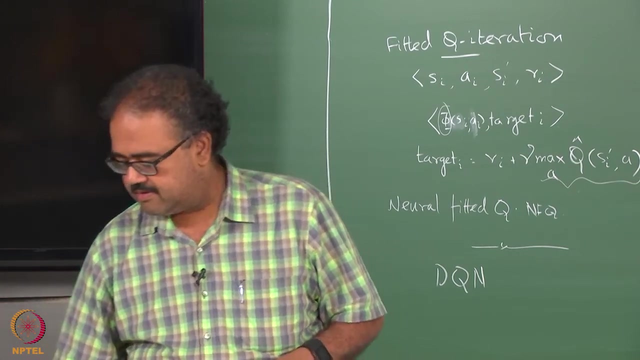 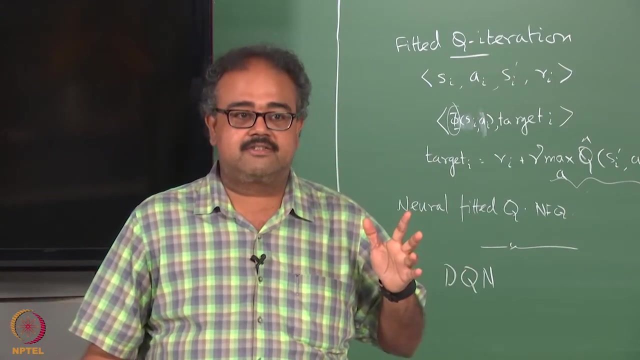 I am sampling g. So what are g's, the returns? so do I know of a way of getting an estimate for g that has a low variance? close value functions. value functions are the expected values of these gradients. this is the g's. 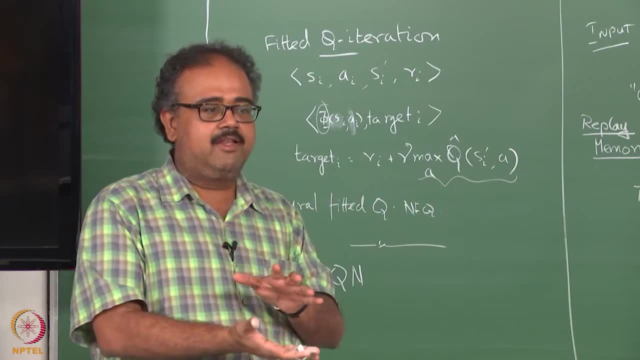 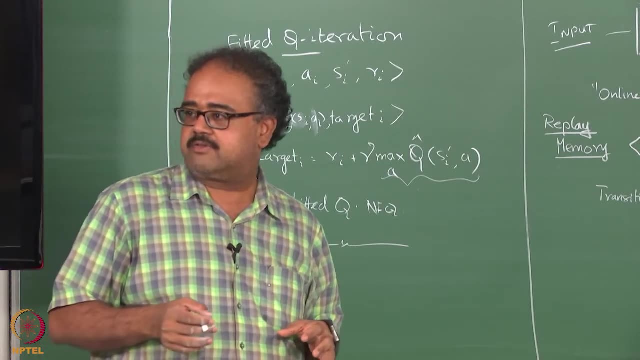 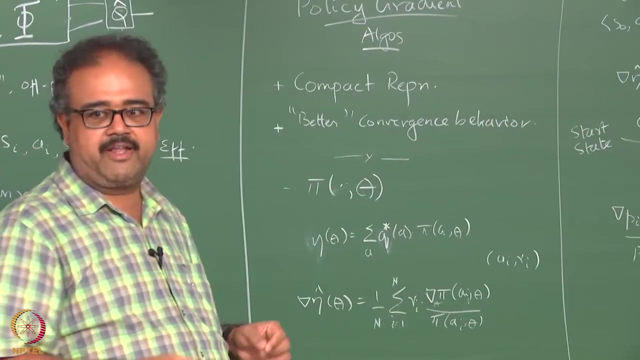 If I know value functions Then I have a low variance estimate for the g's because every time I do not have to draw the sample, I can look at the average of the samples I have drawn so far, and so on so forth. So if I can plug in the value function instead of g some function derived from the value. 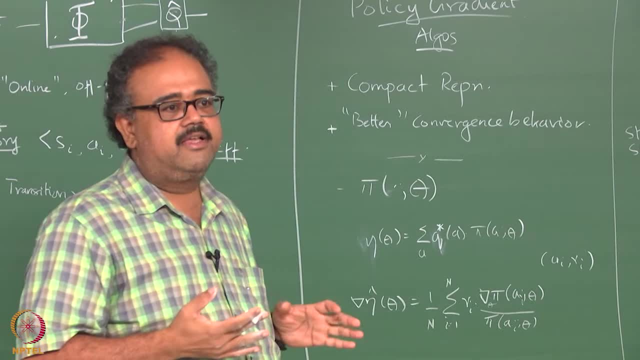 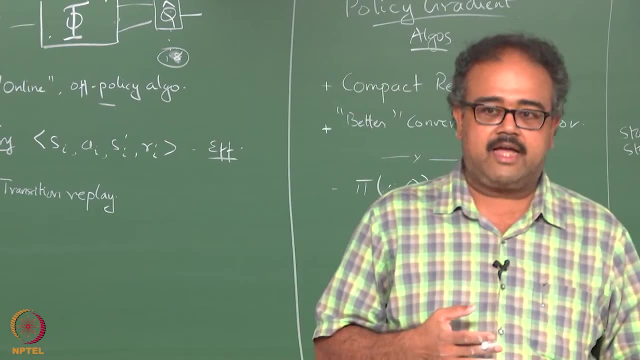 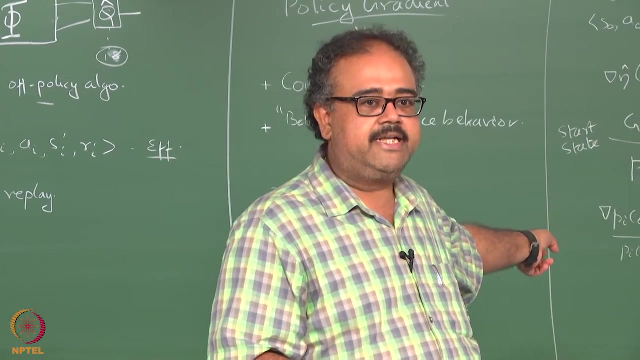 function instead of g's, I can reduce the variance of the updates. I am making variance of the estimates of the gradient. So that leads us to what are called as, after, critic methods. So the actor is the pi representation, the theta gives me the actor. the critic is the. 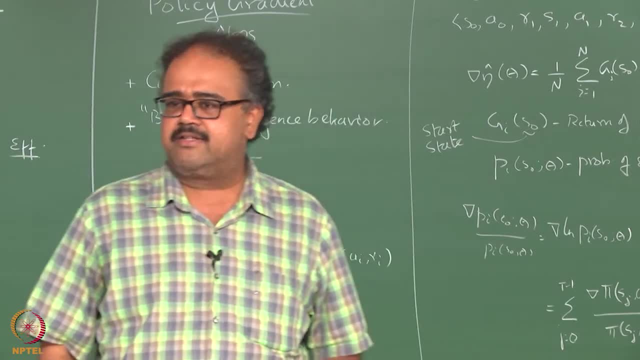 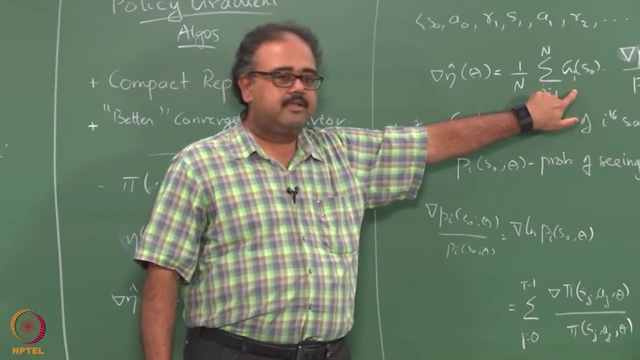 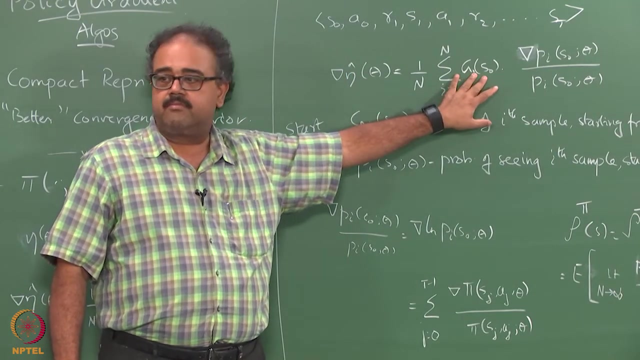 guy who evaluates these actions. he is the guy who says it is good, bad, it is the critic. the critic is the guy who I will plug in here. So the critic is used to evaluate the actor, and the critic comes from any of my favorite. 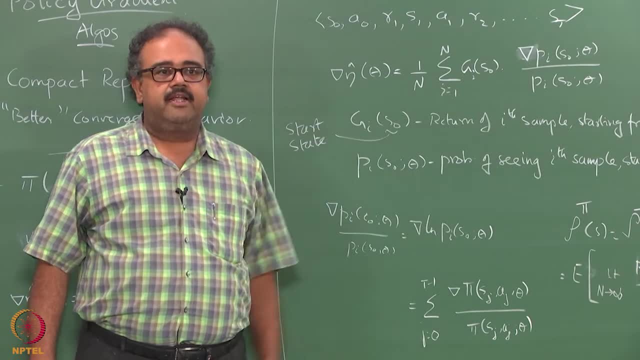 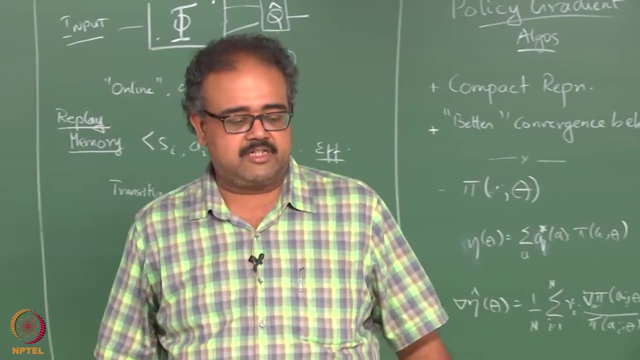 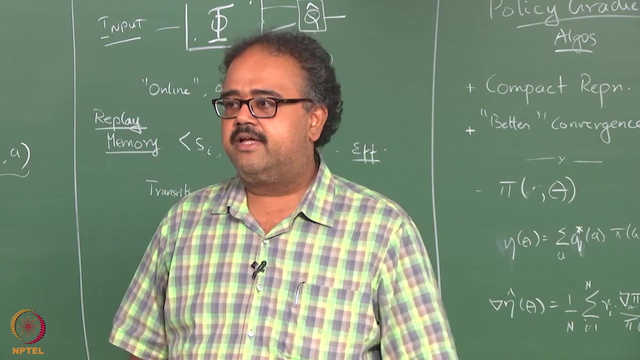 value function estimation techniques. I will typically use a parameterization for the critic as well. I will use some function approximation for the critic and that function approximation will feed into the actor function approximation. I will estimate the actor based on that. So these are called actor critic algorithms. so I will look at actor critic algorithms. 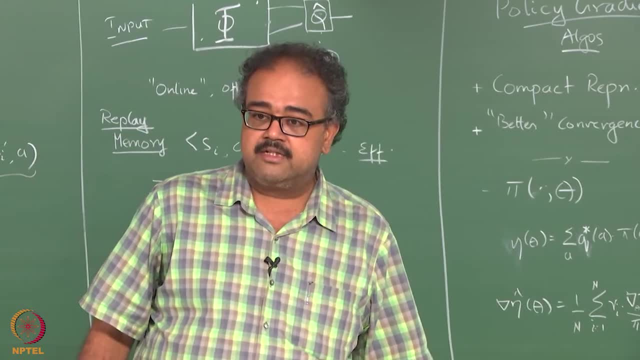 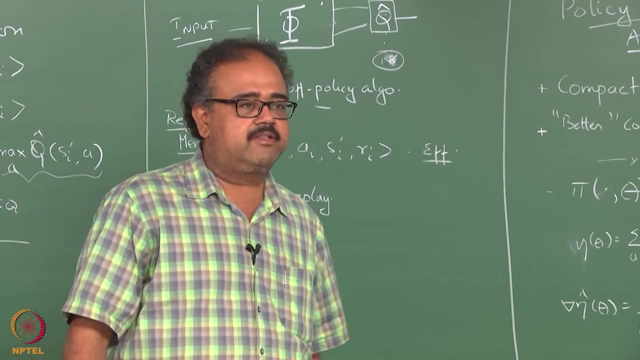 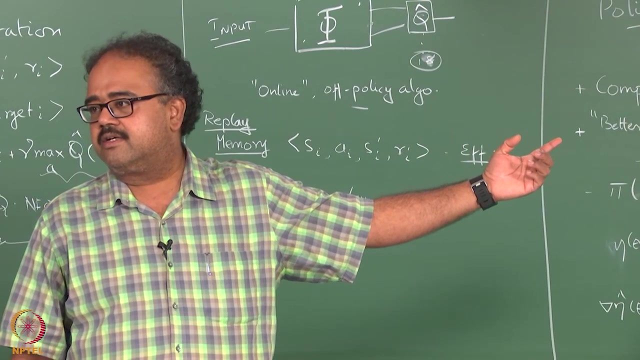 later, possibly in the next class. but basically, I have told you what is the idea behind actor critic. Now, only the nuances that we will have to think about are: how do I actually write this in terms of the value function? how do I take out the return and replace it with the value? 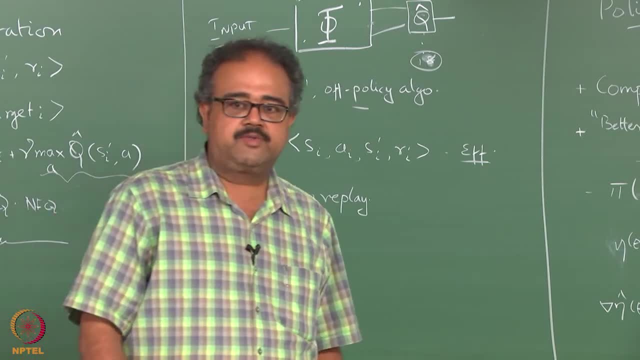 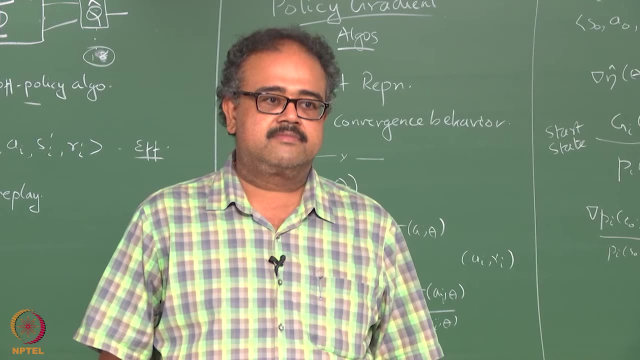 function. So that is the only thing that we need to think about, as well as there are some technical conditions on the relationship between the parameterization of the actor and the critic. I am going to use some function approximator for the actor: some function approximator. 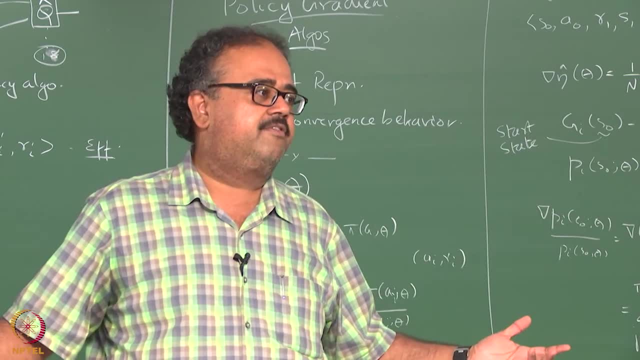 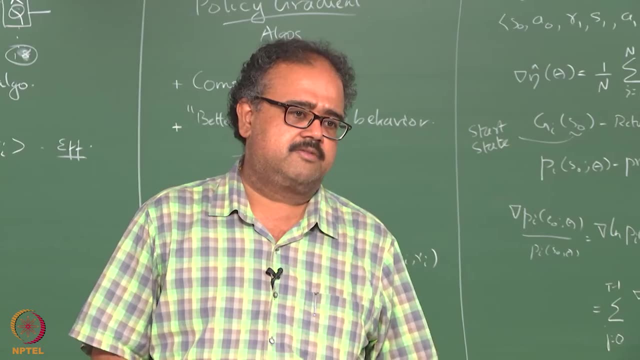 for the critic, And they cannot just be arbitrary function approximation. there has to be some kind of a connection between them. So these are the two things that you really need to think about. so we will worry about this in the next class, but right now I will stop here. Thank you.